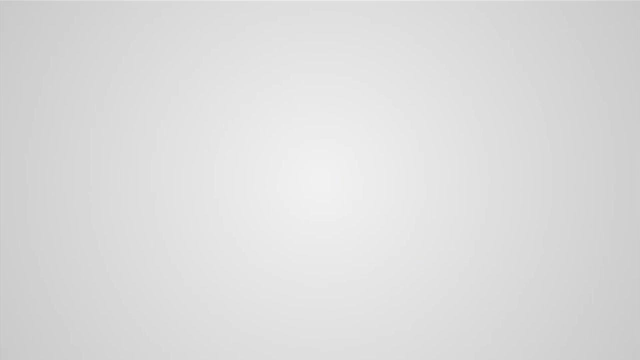 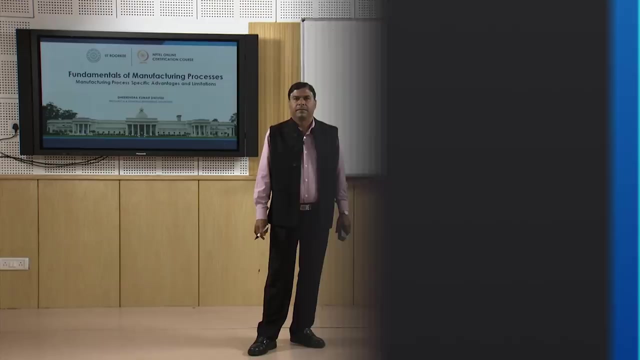 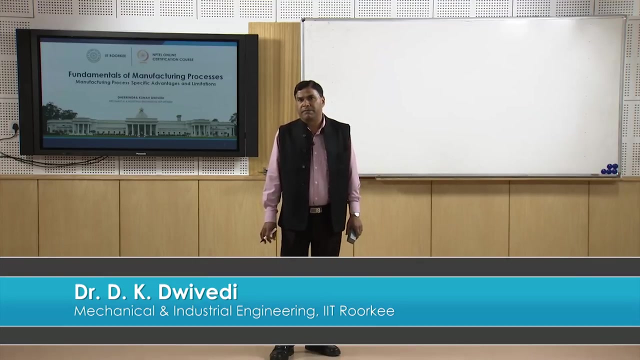 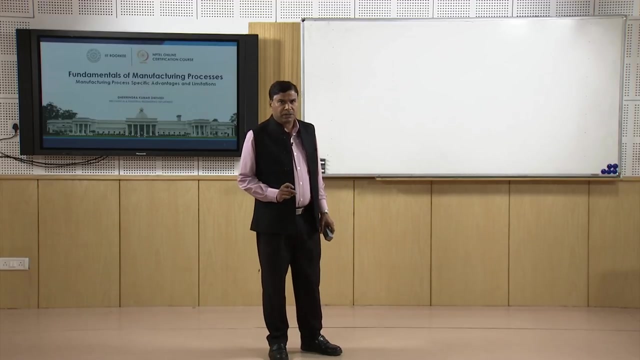 Hello, I welcome you all in this presentation. This presentation relate to the subject of fundamentals of manufacturing process. This presentation is based on the advantages and the limitations of the manufacturing process and the process. specific advantages and limitations we will be talking about here. So we know that the one of the means the most 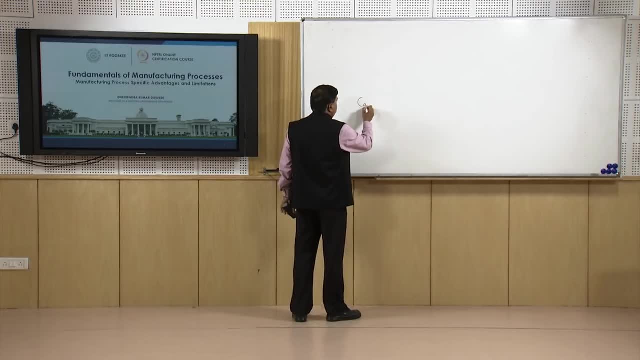 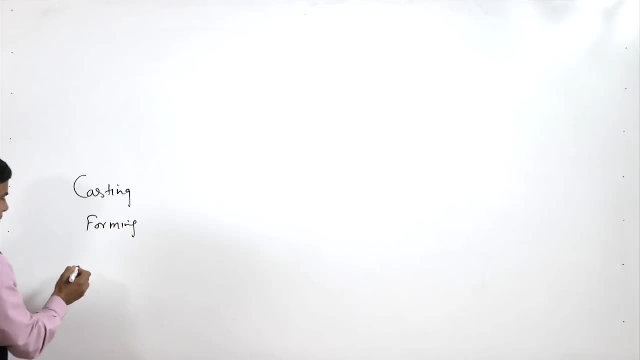 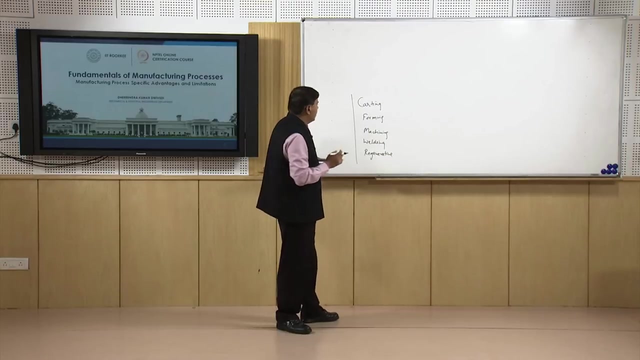 common manufacturing processes include, like casting process, forming process, which are deformation based machining processes, welding process and regenerative processes. So these are very broad group of the processes because in each of the category we have a large number of the processes. These are, you can say, the broad group of processes. 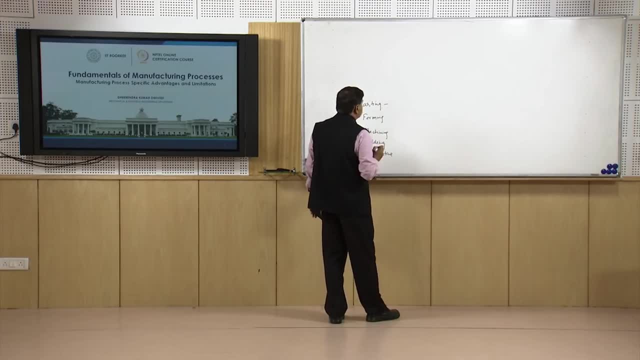 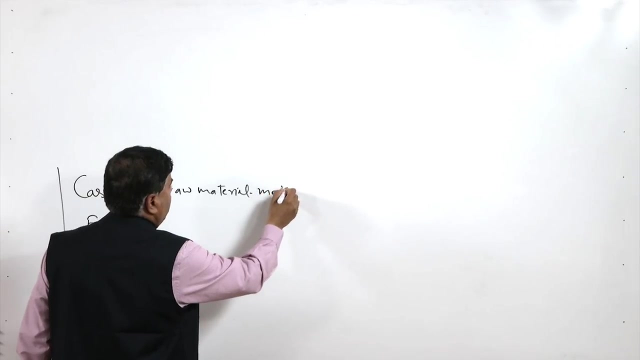 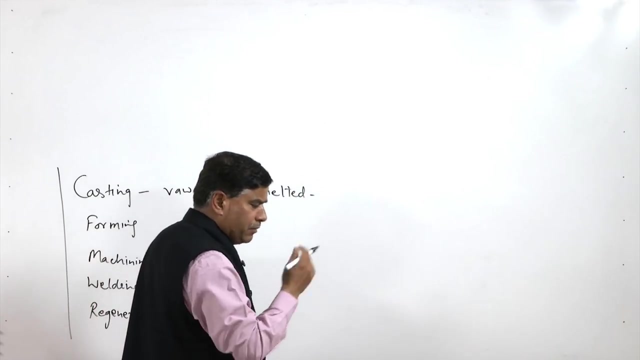 the processes, In casting processes, what is needed to manufacture a product that first the raw material is melted and then to clean the impurities from the molten metal, like the treatment of the molten metal is carried out, where in like degassing, fluxing, etcetera kind of treatment which are 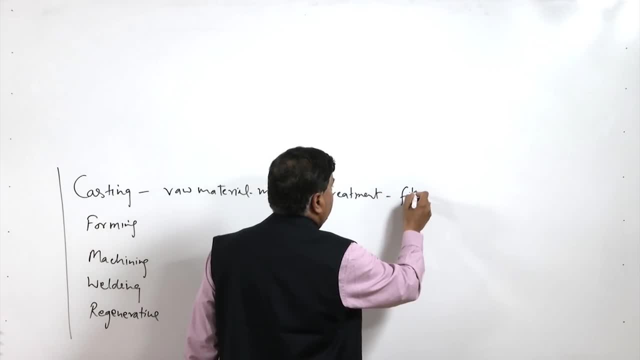 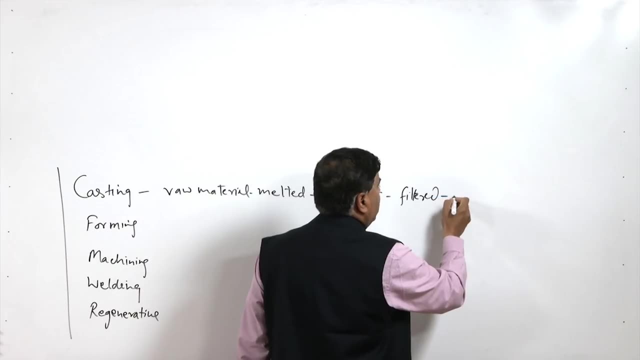 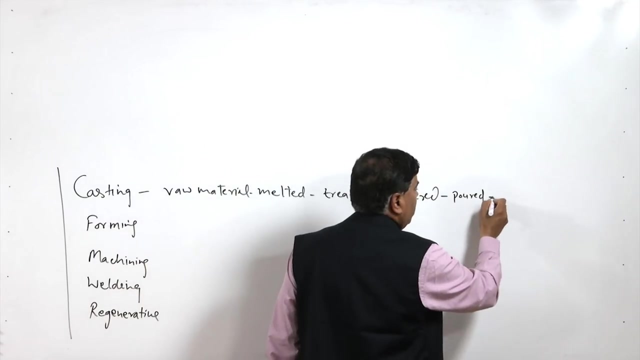 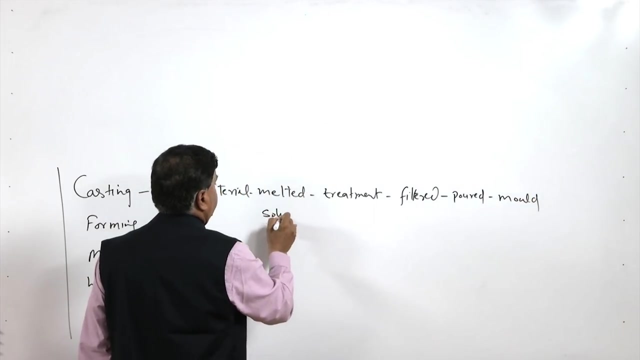 done. Thereafter, impurities are filtered if they are present. So filtration is another step and then filtered molten metal is poured into the mould. So pouring of the molten metal into the mould, followed by pouring into the mould And then the solidification of the molten metal results in the casting and once the 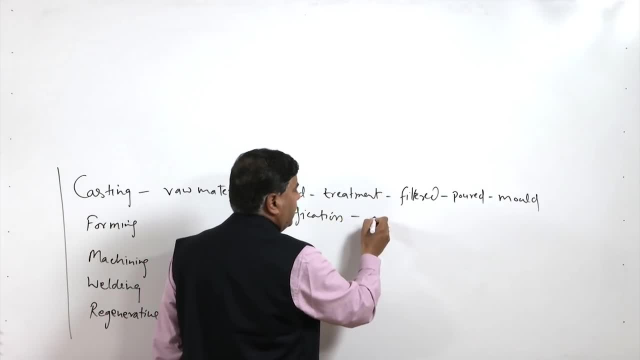 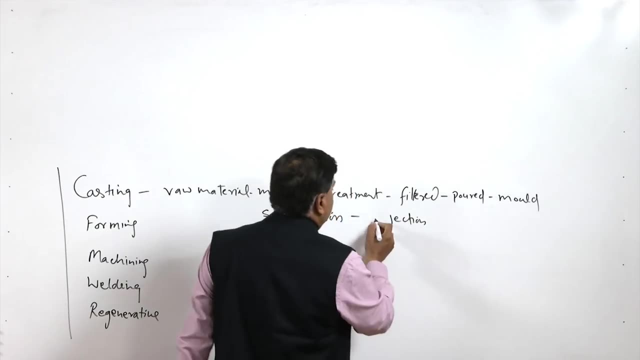 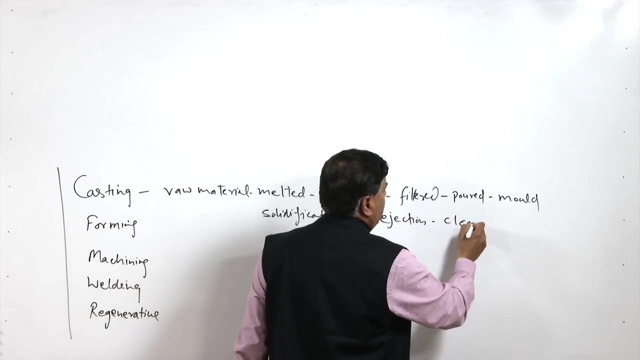 casting is solidified, it is taken out. rejection, or you can say ejection, not rejection, ejection from the mould and then cleaning and fettling, etcetera, as per the process. Thank you. Thank you, That is the process which is done. 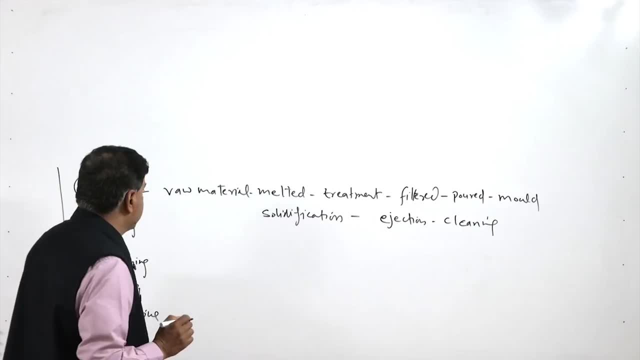 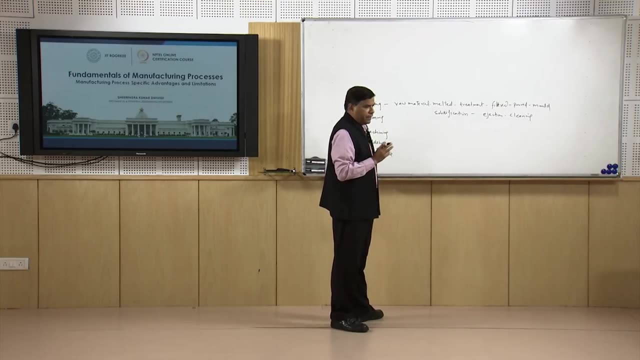 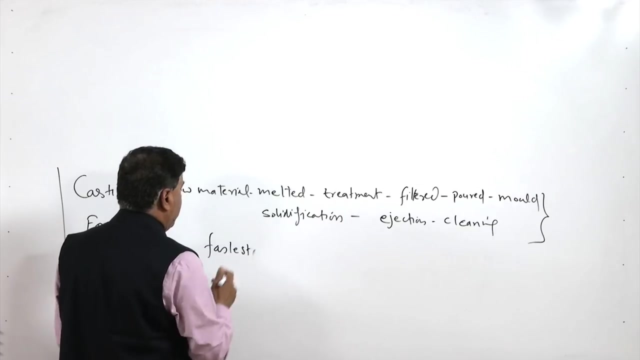 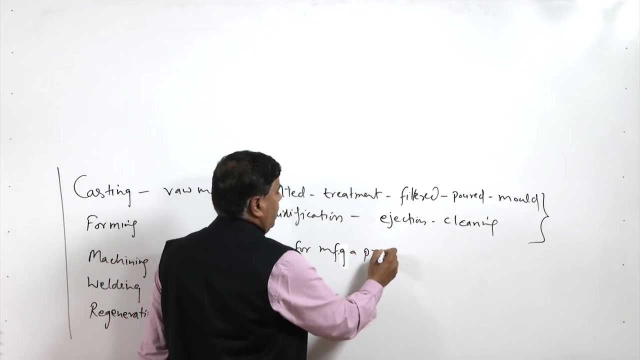 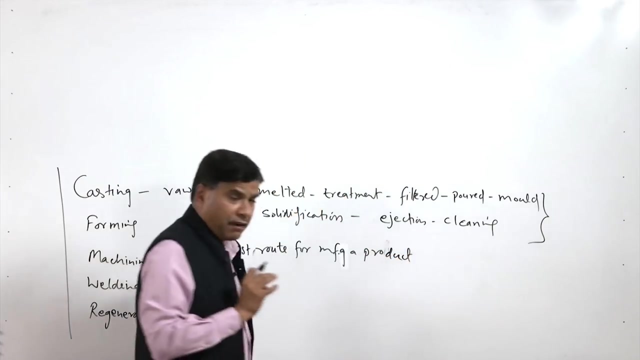 So, if we see this process, this process, these are the steps and, from the capability point of view of this process, this process can, this is, this process offers the fastest route, fastest way or fastest route for fettling route, for manufacturing a product or to get the desired shape, but the surface finish. 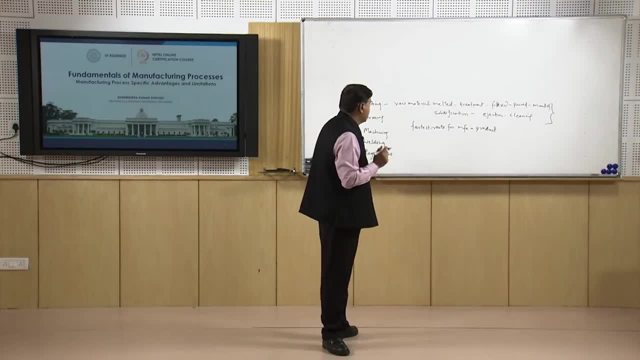 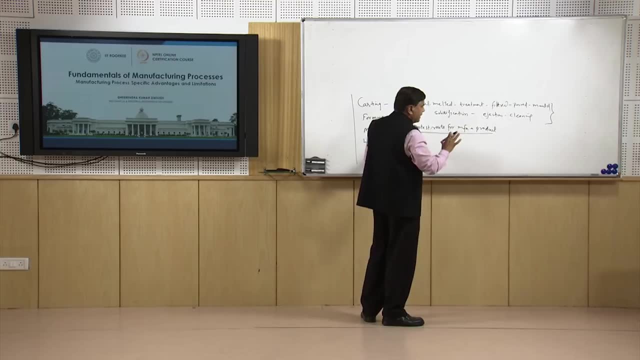 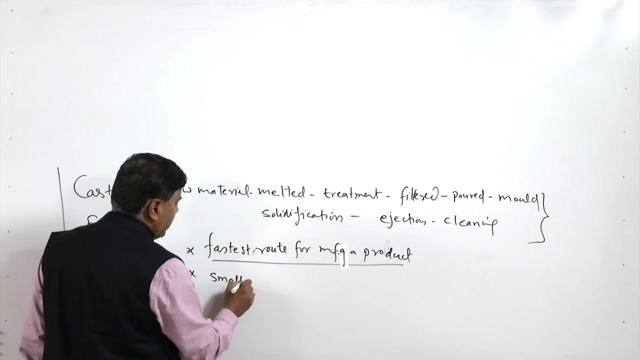 and the tolerance which are achieved by this process are not good. So this is the fastest route, because we melt and we get the desired size and shape, but the finish and the tolerance which is achieved is not very good. This casting can be used for making the products of very small size, maybe of a few grams to 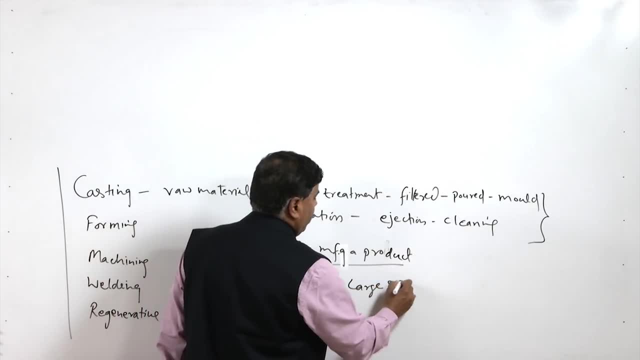 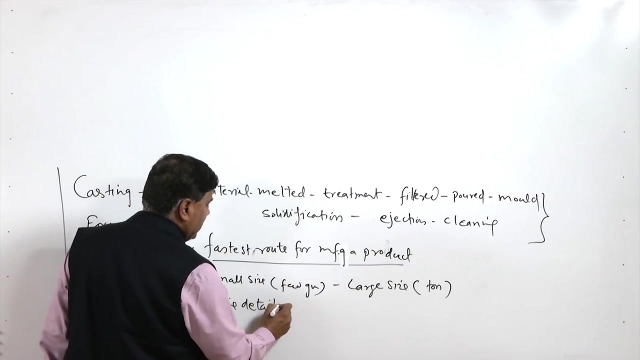 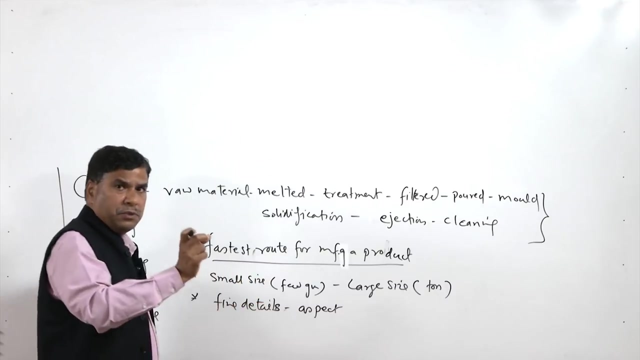 the very large size, maybe few tons, also like 100 ton, 200 ton castings are also made, And very fine details can also be achieved. fine details in the products can be realized, and so the quite good aspect ratio means the height to the thickness or the width of. 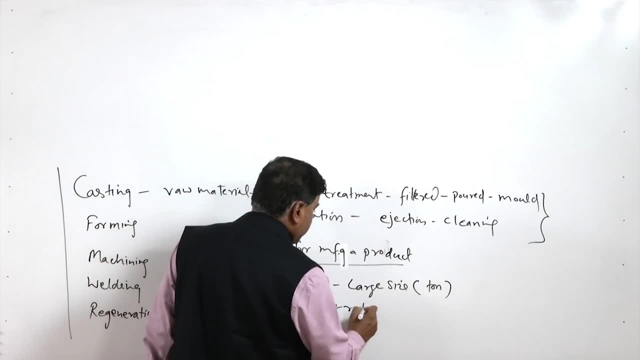 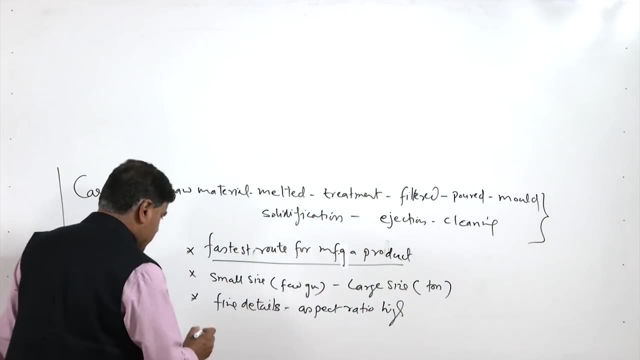 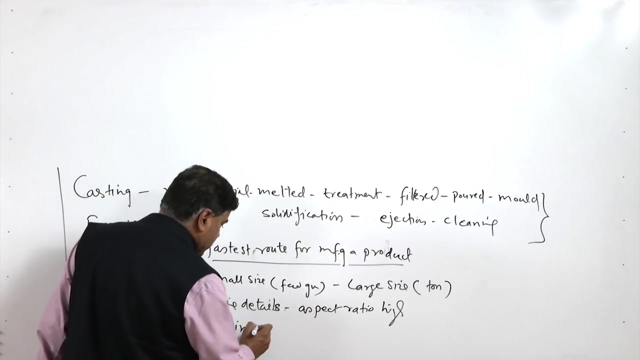 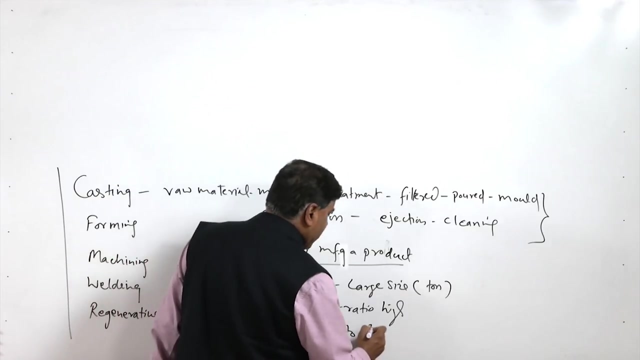 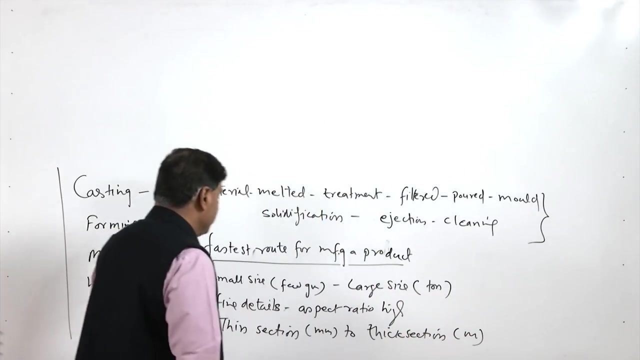 the slots and the groups which can be achieved is very good. So aspect ratio which can be achieved, We achieved- is also high. so means we can say it can be used for the making components of very thin sections of few mm to the very heavy thick sections, maybe in meters also. 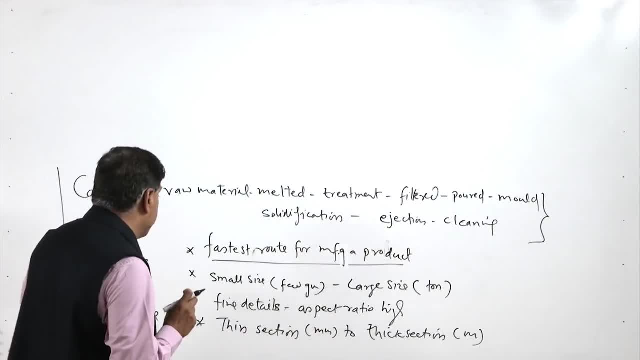 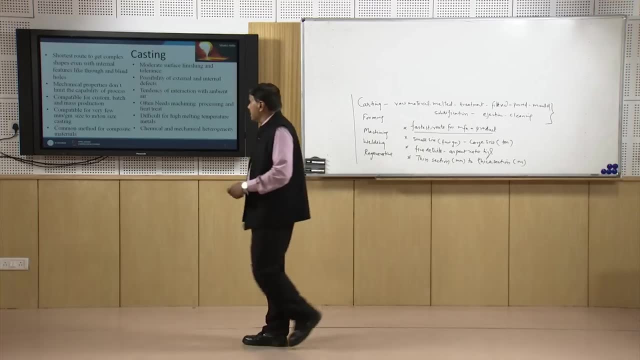 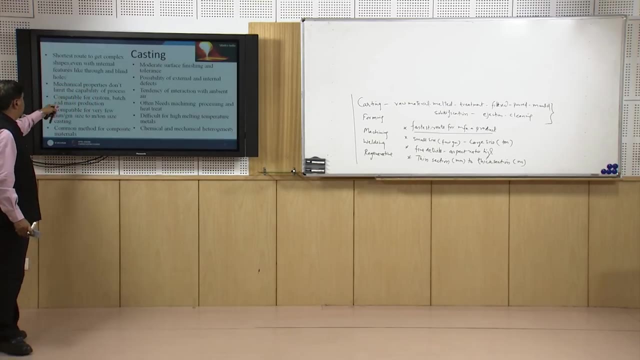 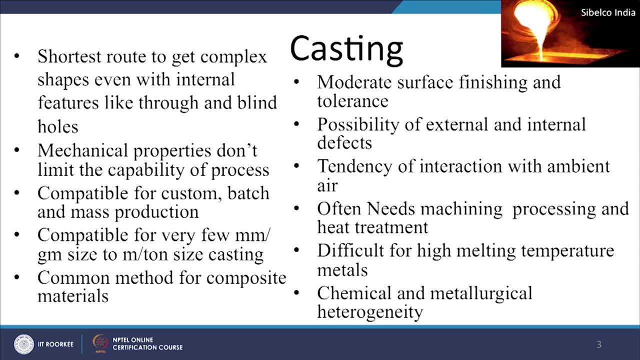 So these are some of the very positive sites Related with this process. to see more details related with this, this process offers the shortest route for manufacturing a product, like shortest route to get the complex shapes with the internal features through holes or the blind holes or any other geometry of that. 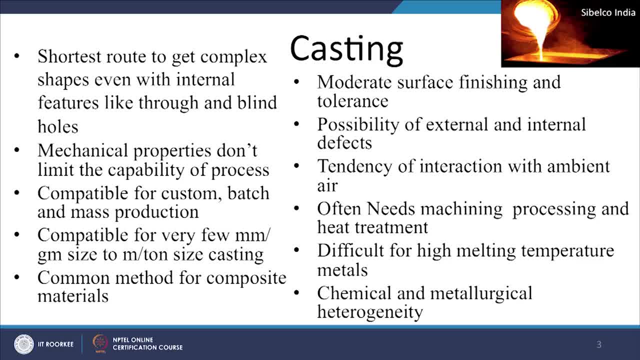 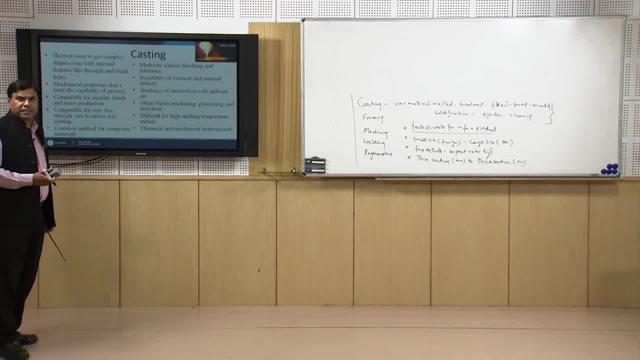 kind. Another important thing: mechanical properties of the material do not affect the success of this process, The more because, whether it is material is hard or tough, or very strong or very low ductility or of very high ductility, that does not affect the processing capability of the casting to 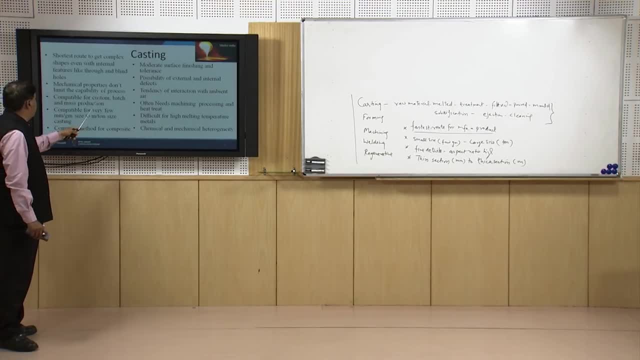 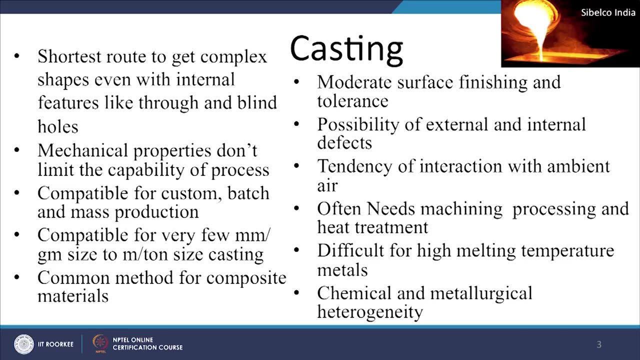 get the desired size and shape. So mechanical properties do not affect or do not limit the capability of this process and compatible for custom batch and mass productions. So this is important. we can make a very large size casting in a single casting of very large 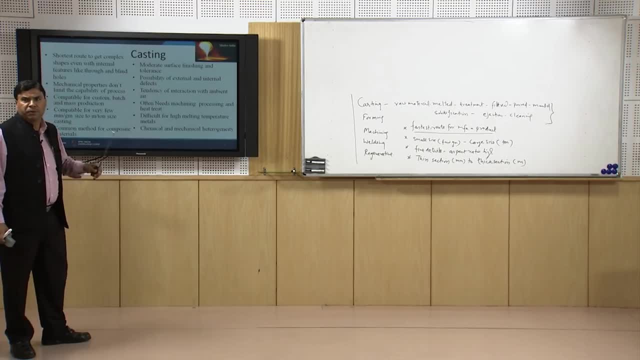 size or we can make few number of components, like a batch of 10 or 50. number of products can be made by the casting economically. at the same time the process can also be used for the mass production purpose. So that is the Another good feature related with the casting. that process is compatible for the custom. 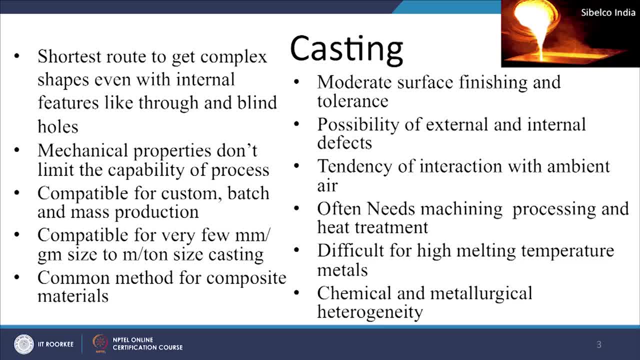 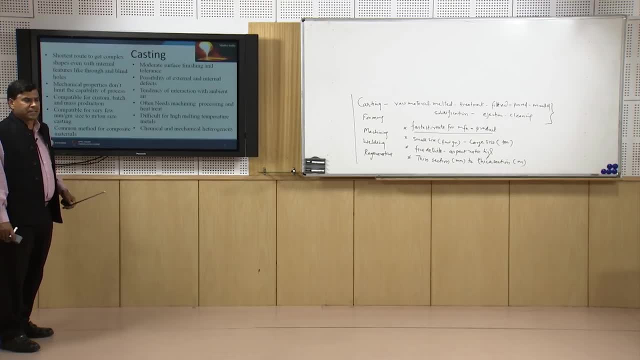 made products or customized products, or for the batches of the different sizes and for mass production purpose Like this process is therefore very commonly used in the casting in casting industry for making the wheels, for making the piston rods, case, engine blocks, etcetera and the compatible. 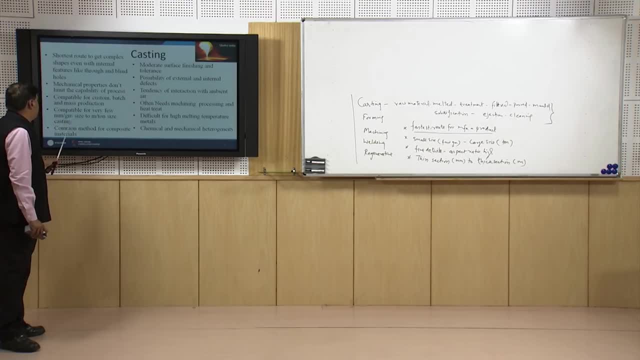 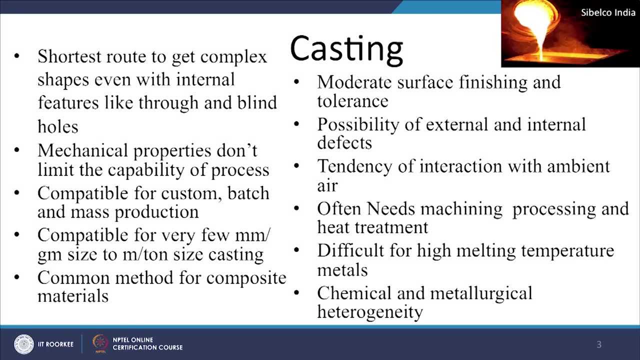 for very few of for very fine dimensions to the very large size dimensions like, say, the components may be of very small size in mm, or sections may be of very small size in mm, or a very large size in meters or in tons, and this is common method for making. 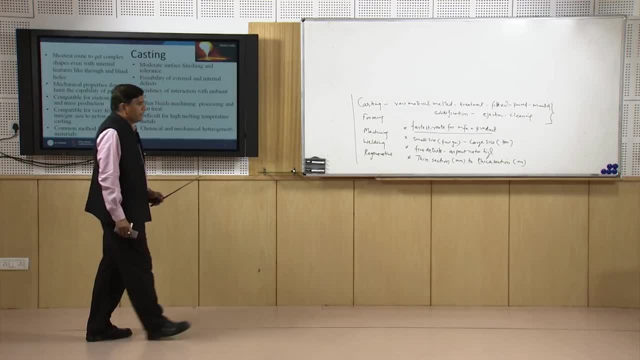 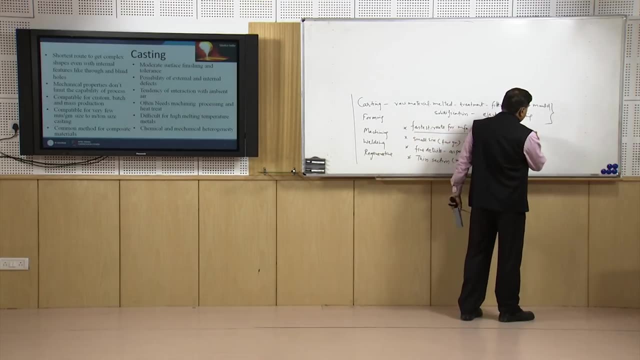 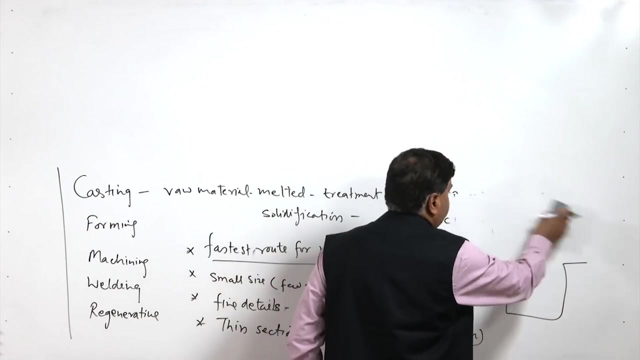 the composite materials. also, like the stir casting or rio casting, is one of the route where So the molten metal, where casting is used for preparing the composite materials. So in this method, what is done? basically, the molten metal is maintained at a correct. 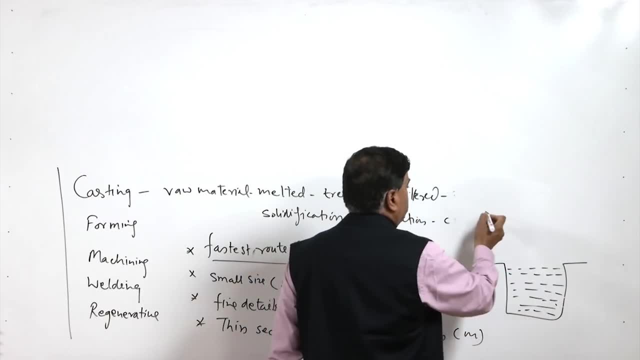 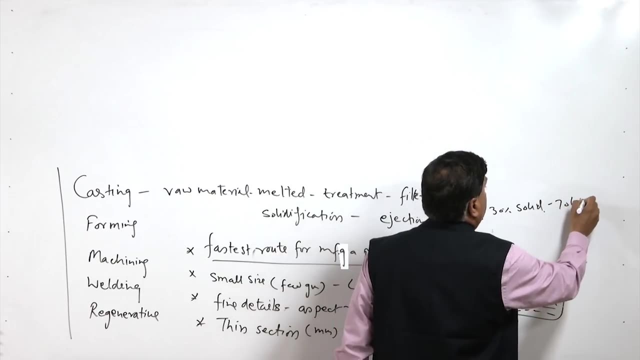 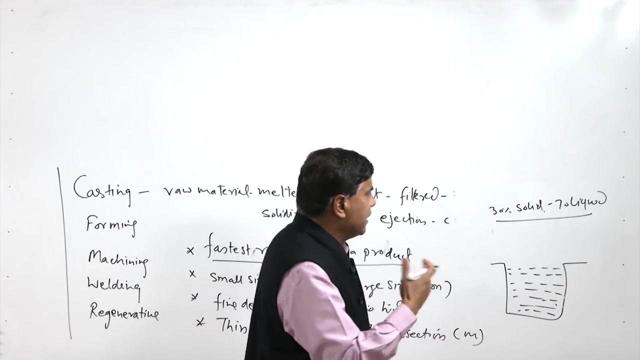 temperature, So that there is a mushy zone wherein like, say, 30 percent solid and 70 percent of the liquid. So this is the two phase A state state normally used, like 20 to 30 or 40 percent of the solid and the remaining liquid. 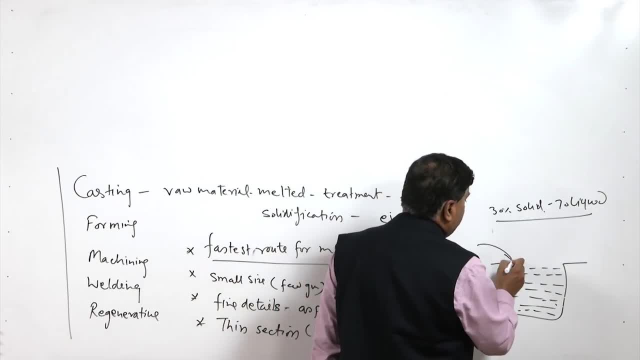 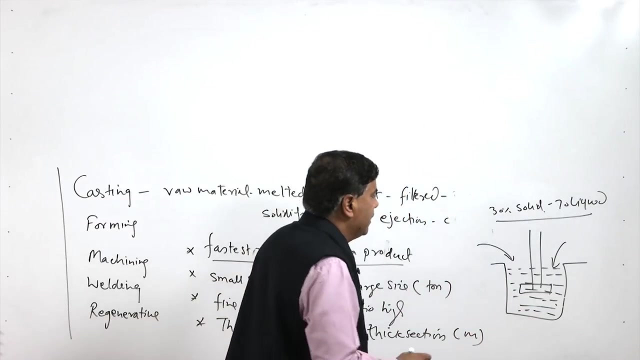 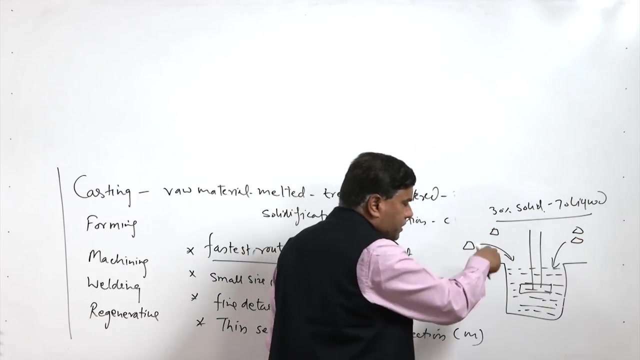 So in this condition the particles that we want to reinforce in the casting they are fed in with the help of a stirrer. this molten metal is stirred and then we feed in the ceramic the particles or any other particle which is to be reinforced so that it gets distributed. 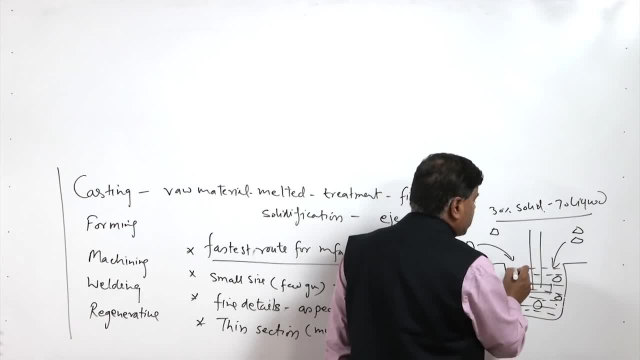 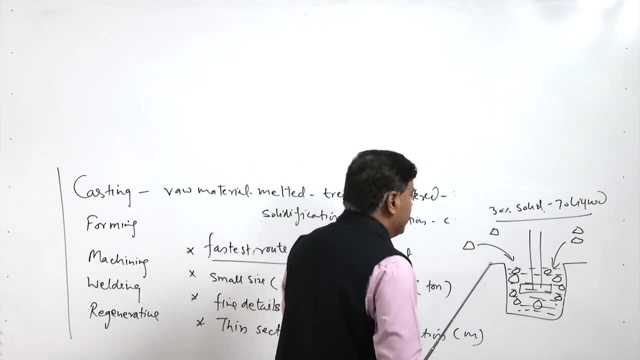 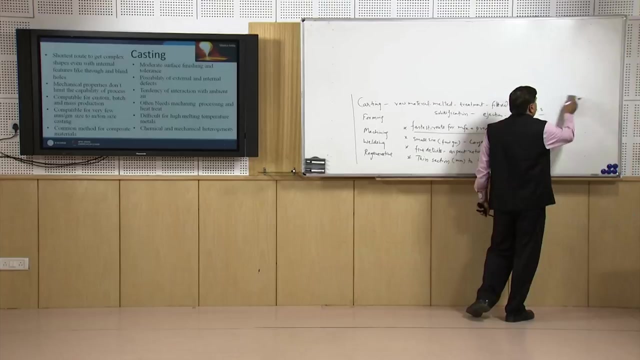 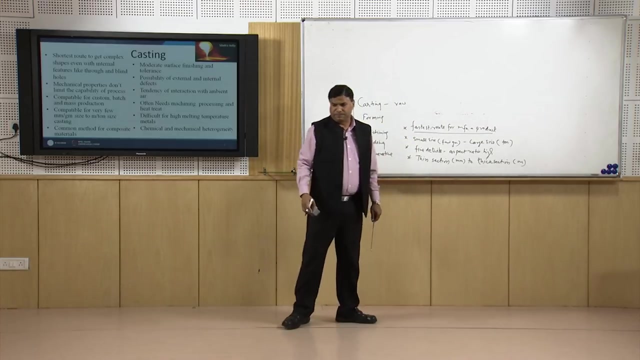 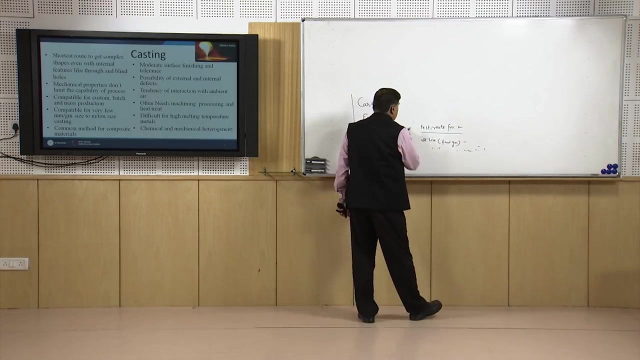 into the mass or in this semi solid metal and then it is allowed to solidify, and that is how this casting is also used for making the composites. All the composites can be made using other routes, like the powder metallurgy, And there are various methods for making the composite materials. 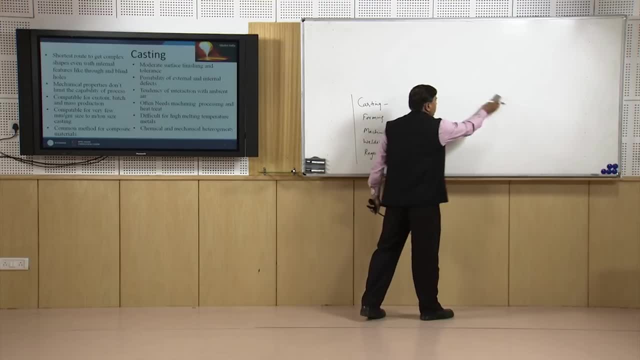 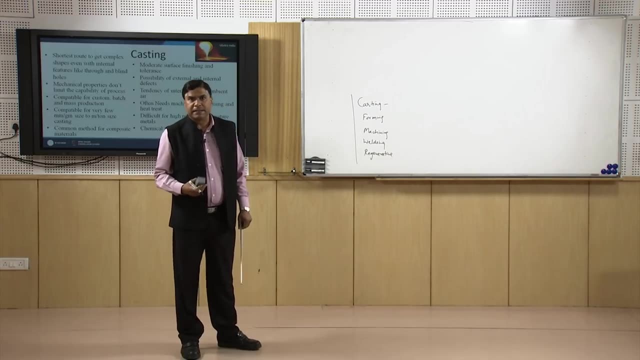 Now coming to the limitation of the process. the limitation is that it is required that for this process it is necessary that the material is brought to the molten state. so melting of the material is mandatory and for that purpose it is necessary that the melting 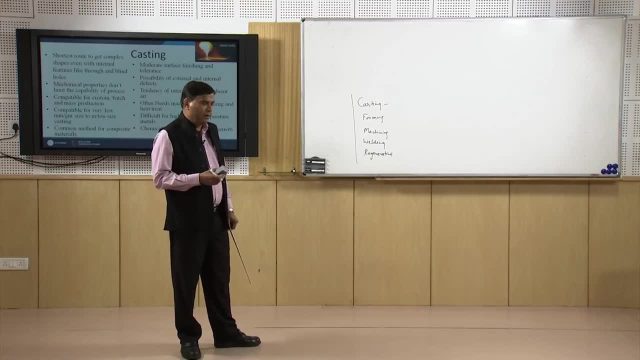 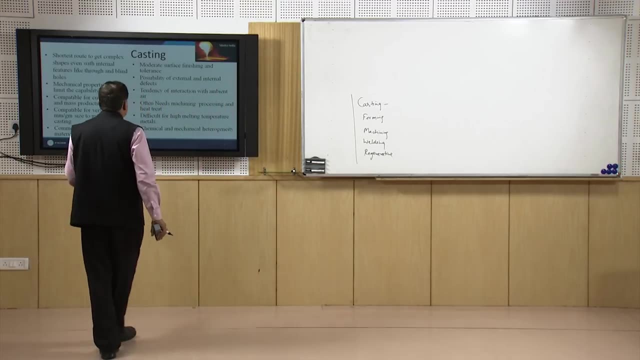 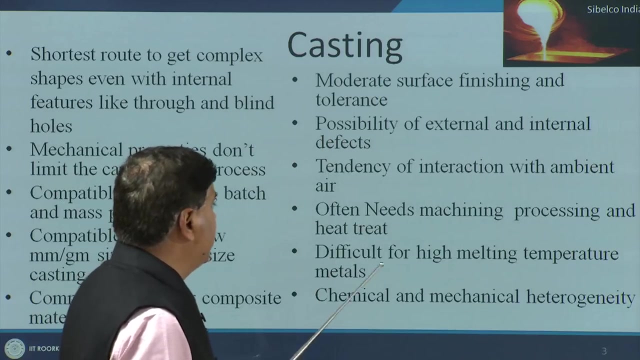 point of the material must be reasonable, Reasonably low, or if it is too high then it will make the melting of the material difficult and that is why the high melting point materials are found difficult to process, to be processed by the casting process, like difficult for high melting temperature metals. 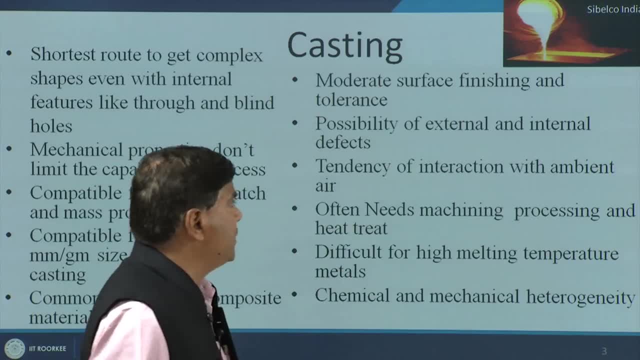 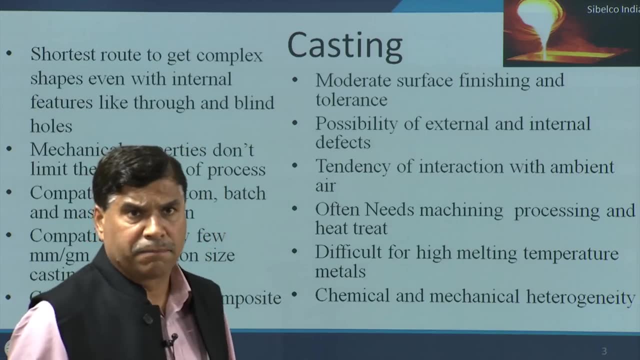 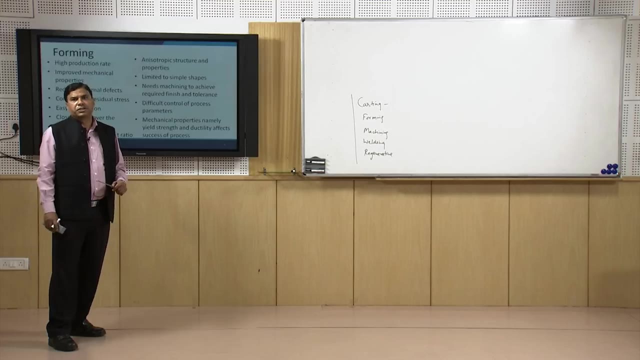 And, at the same time, the surface finish which is achieved by the casting process is not that good. It requires a secondary process, It requires a secondary processing in form of the machining and, at the same time, tolerance is also not good and therefore, to achieve the close control over the dimensions to have, 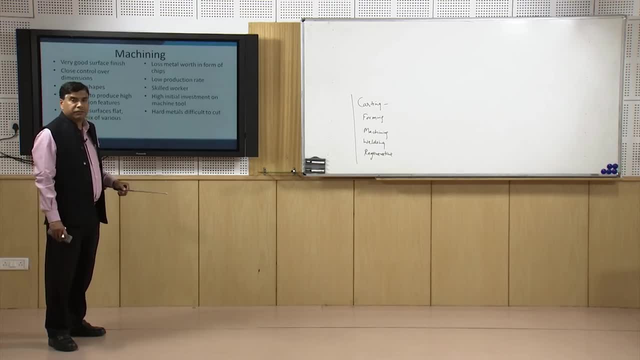 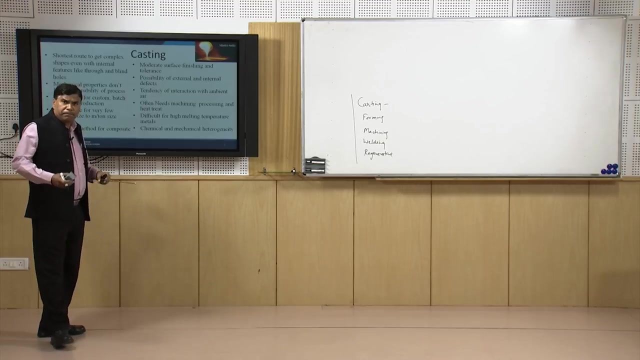 the close control over the tolerance of the manufactured product, the machining becomes important as per the requirement. Then the possibility of the internal and external defects. we know that the molten metal will be solidifying, So if the gases remain, get trapped or impurities are passed into the with along with the molten. 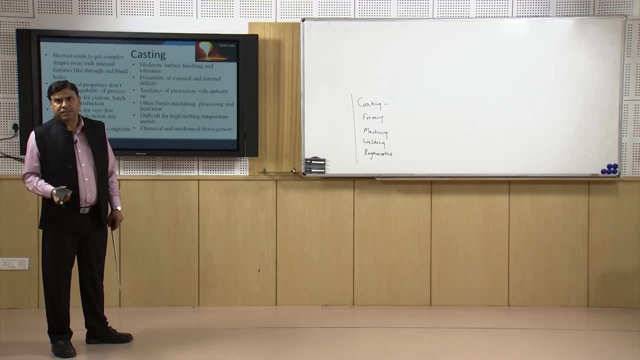 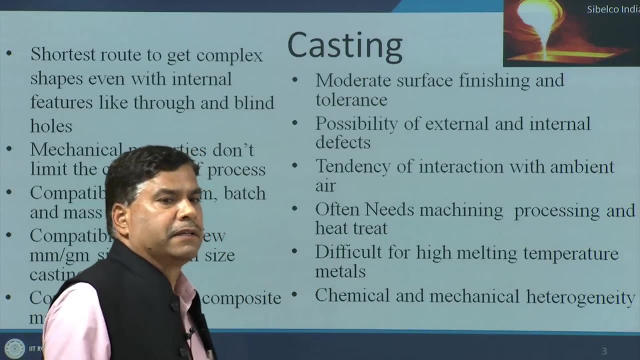 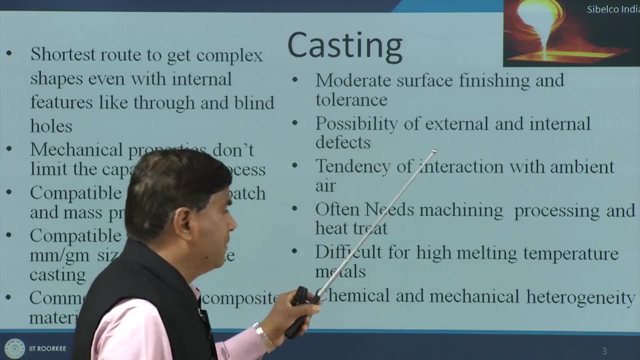 metal they get into the mould, then they will be present in form of porosity or the inclusions, So which will be leading to the internal defects. at the same time, like the formation of the cracks due to the high residual tensile stresses can lead to the development of the 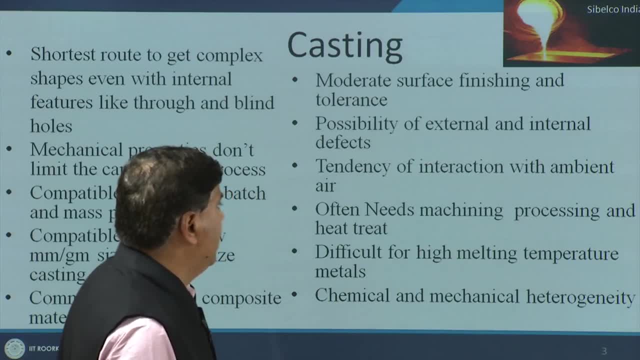 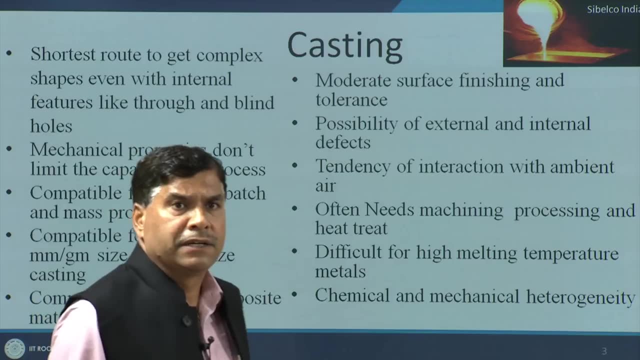 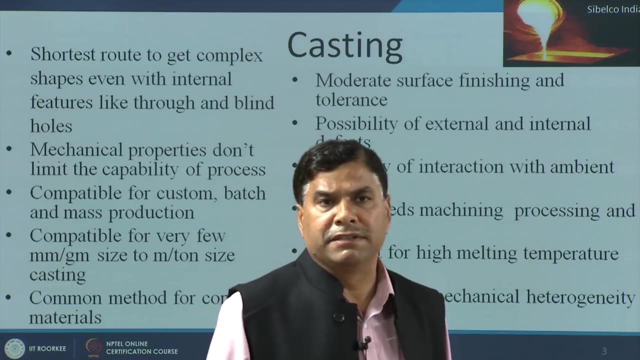 cracks in the surface surface of the castings and, another important thing, tendency of the interaction with the ambient air. We know that whenever the temperature of the metal is increased it becomes active to the atmospheric gases and with the increase in temperature it can absorb or it can dissolve. 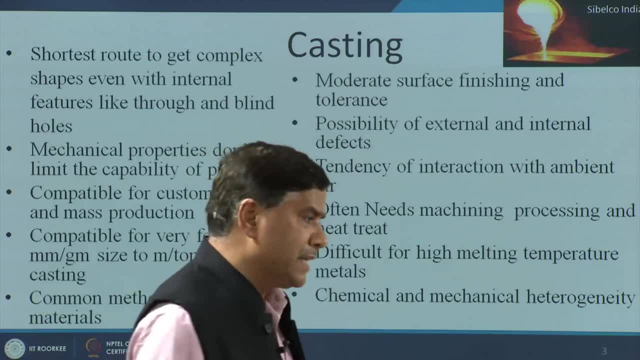 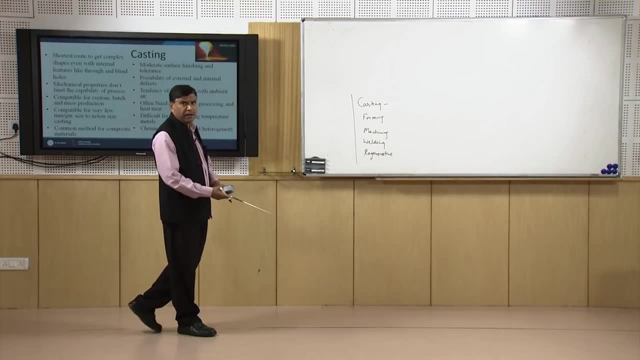 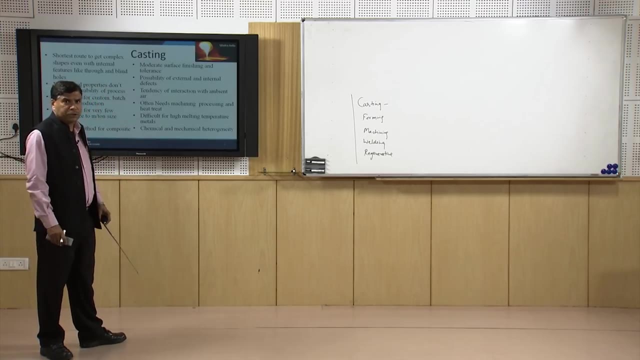 more amount of the gases in the liquid state as compared to the solid state. So the differential solubility in the liquid and solid state leads to the problem of the porosity. if the gases are not, they do not find enough opportunity to come out of the 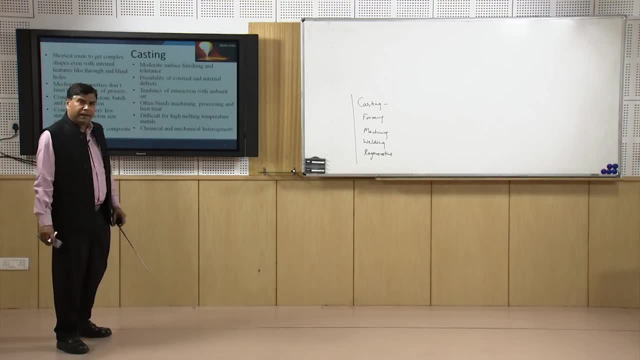 casting during the solidification and these gases also sometimes react with the molten metal and if these do not flow toward the surface of the molten metal during the solidification, then they may get remain So trapped into the castings and that will be leading to the defect. often needs machining. 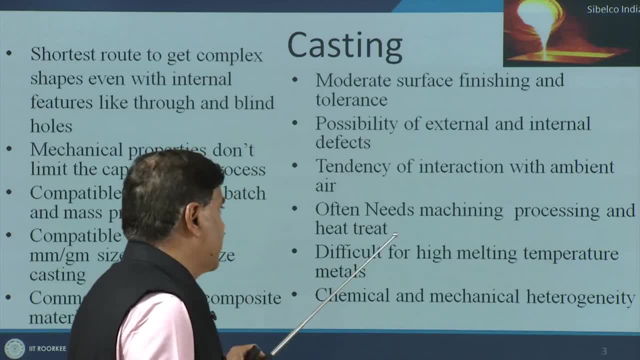 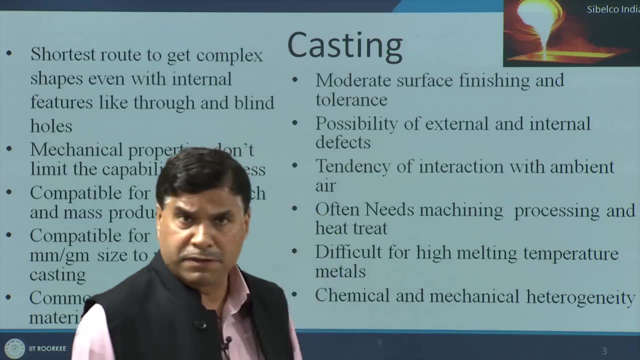 and process machining: process processing of the casting by machining and the heat treatment. We know that since the control over the dimensions and surface finish which is achieved in the casting is not very good, therefore, to achieve the desired degree of surface finish and close control over the dimensions, the machining becomes important, as per the functionality. 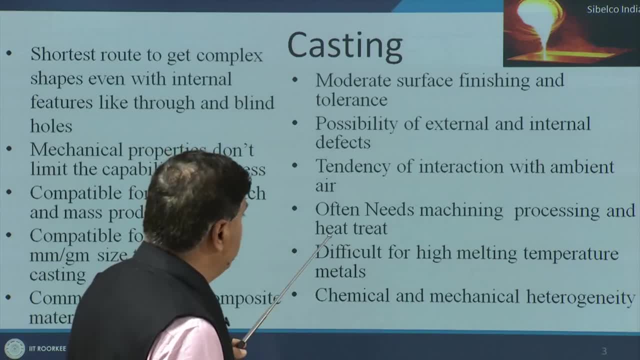 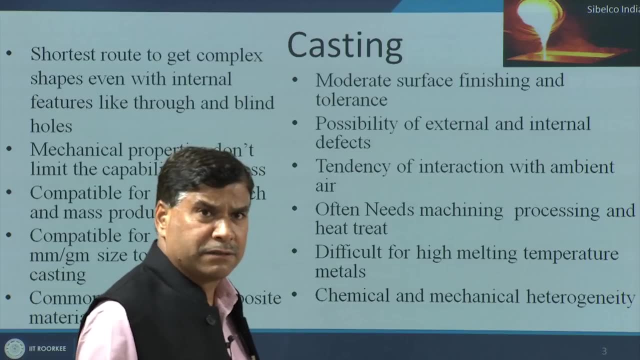 or as per the requirement of the service. Similarly, heat treatment is of the casting is also carried out to enhance the characteristics and properties of the castings because in as cast conditions, casting offer somewhat poor mechanical properties and therefore to enhance the properties of the casting sometimes. 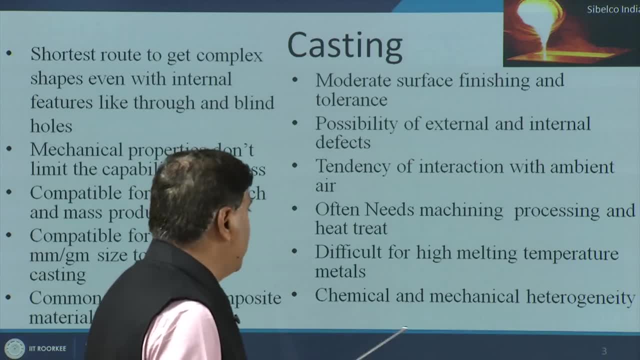 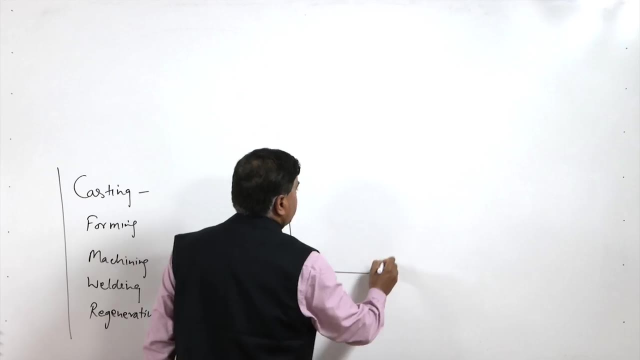 the heat treatment is also carried out and the chemical and metallurgical heterogeneities also exist in the castings. That is another side. Let us look at more of the technological point related with the casting. like whenever the solidification of any casting takes place, we find that the pure metal solidifies fast. 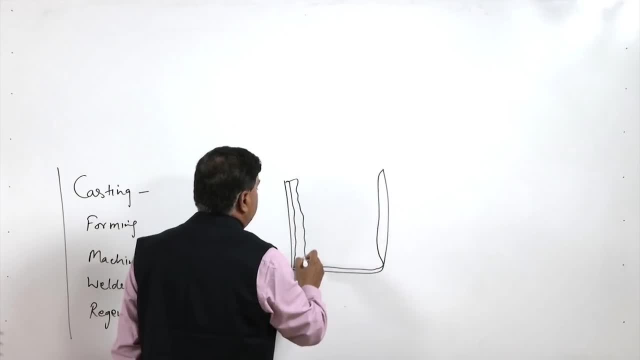 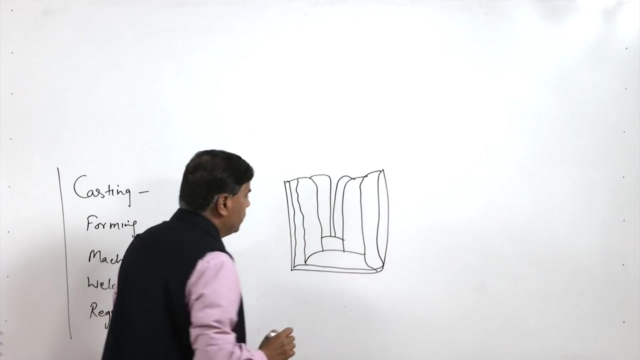 and gradually, the impurities or the alloying elements will be segregating or will be moving towards the centre. and at the end, what we find? that all the impurities have got solidified. 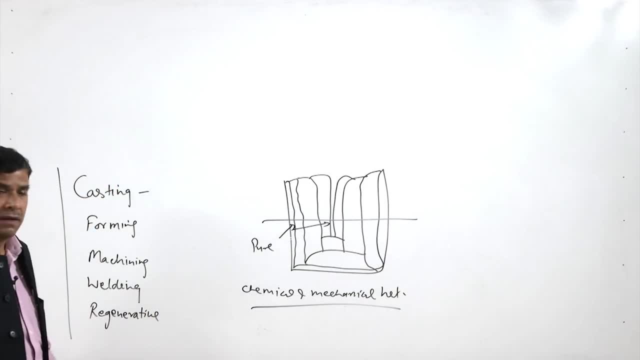 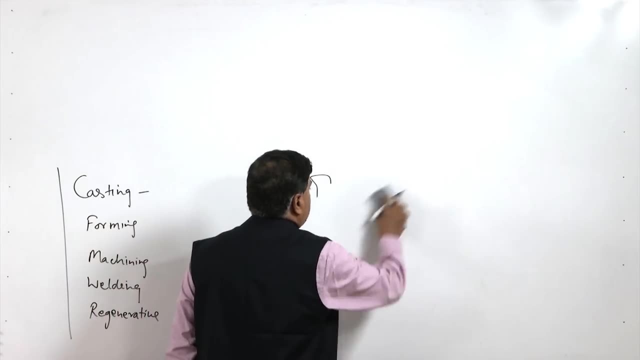 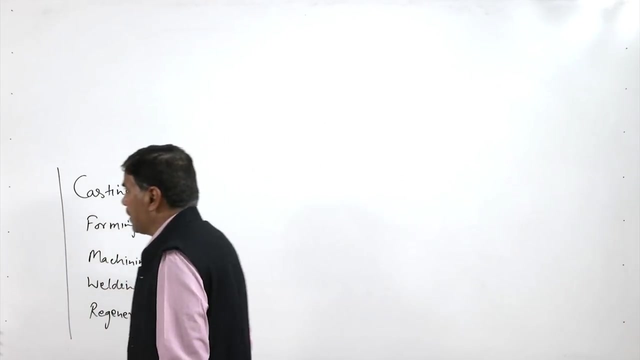 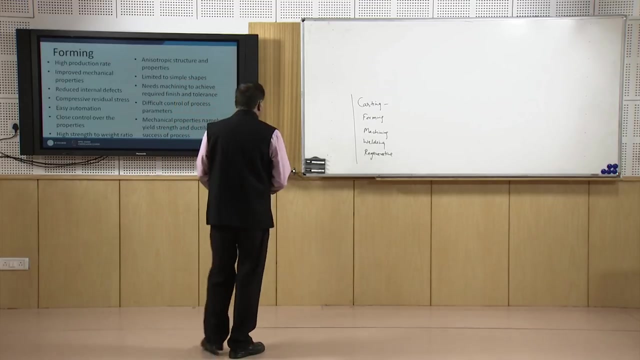 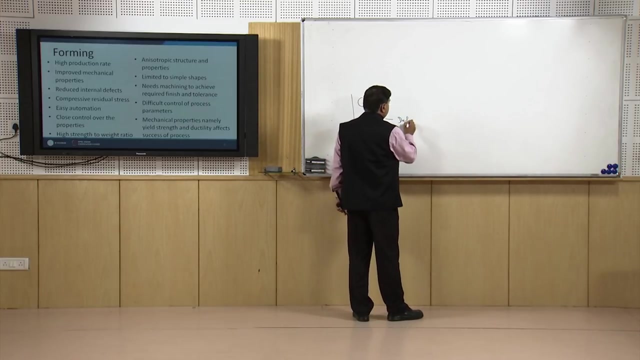 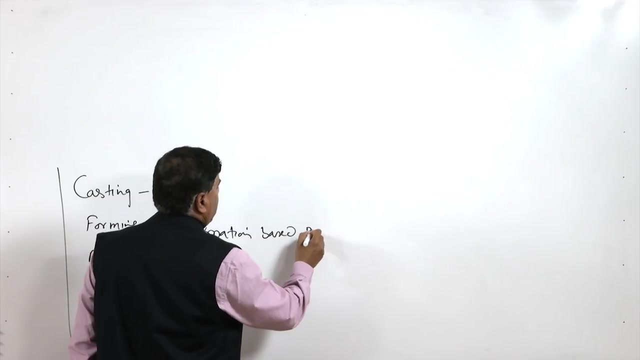 So to. so this is inherent feature of the casting process, where the micro level heterogeneity always existed, and sometimes even macro level heterogeneity is also found in the castings. Now coming to the another process, which is a forming. So, in case of the forming, forming is a deformation based manufacturing process where normally 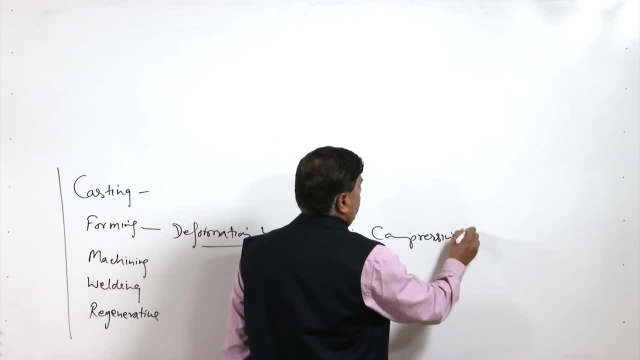 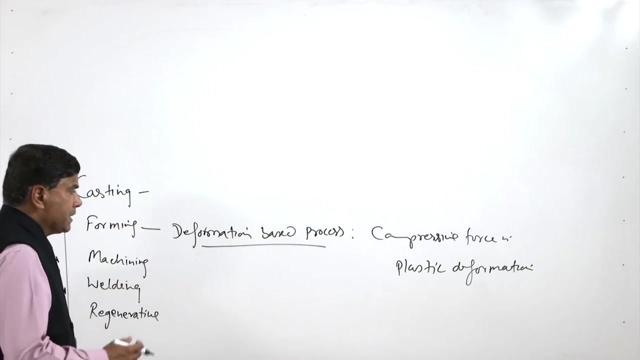 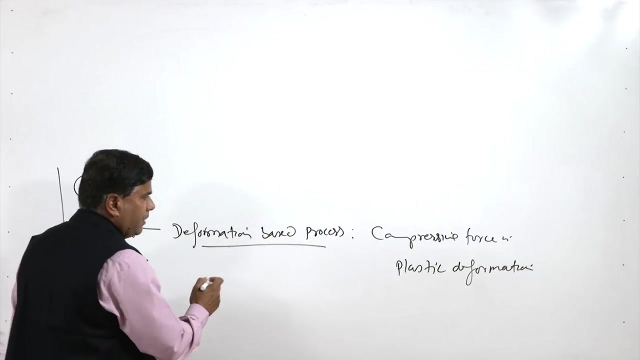 compressive force is applied for plastic deformation and in order to achieve the desired size and shape. but since this process uses the plastic deformation to achieve the desired size and shape And using those, and the nature of the application of these forces is such that it cannot really 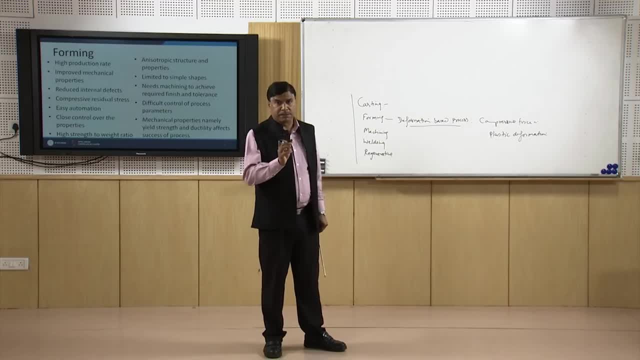 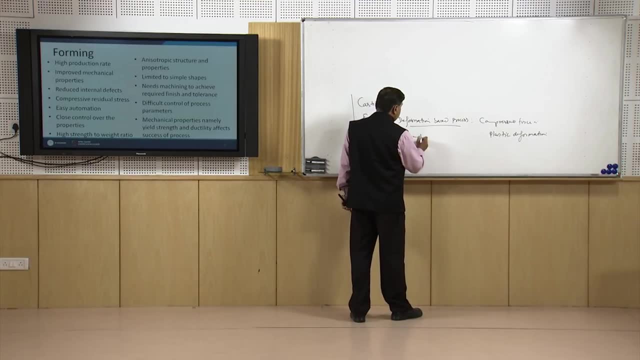 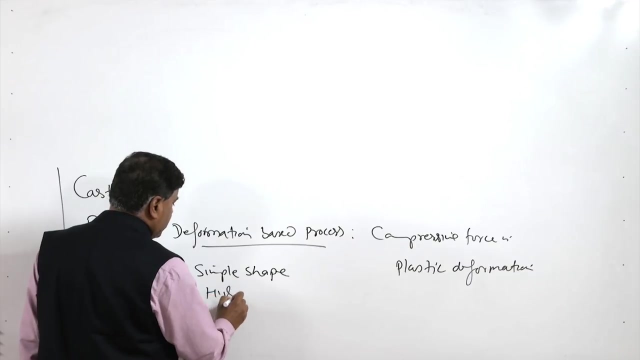 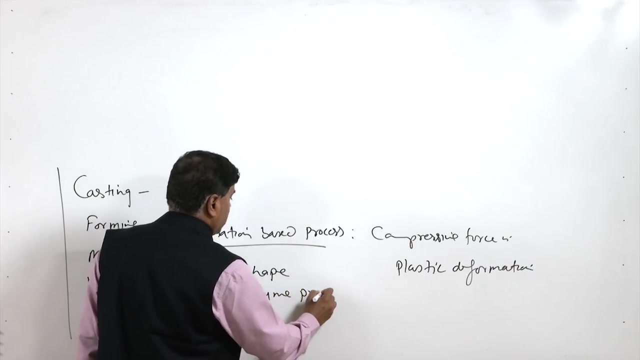 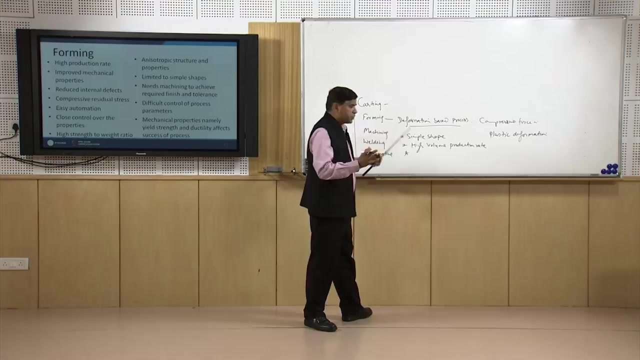 help to achieve the very complex shape, very high aspect ratio, geometries, and therefore this process is found good for simple shapes. This is one this process offers means this category of the process offers the high volume product. This is the production rate generally. the deformation is associated with the closing. 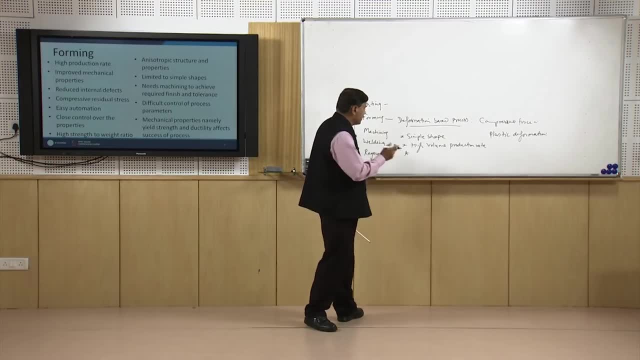 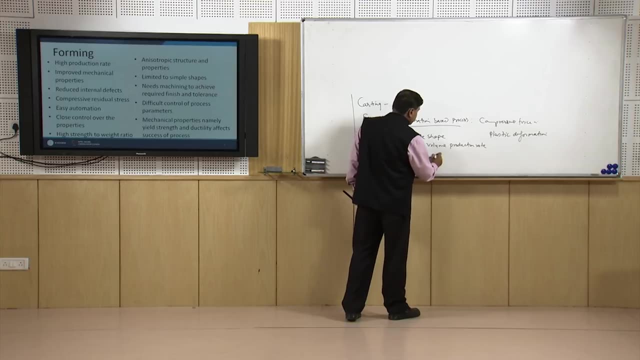 of the discontinuities and the defects if they are present in the material. So basically, it eliminates impurities, defects and discontinuities. if they are present under the compressive plastic deformation conditions, These are eliminated from the drama. So this is the process. 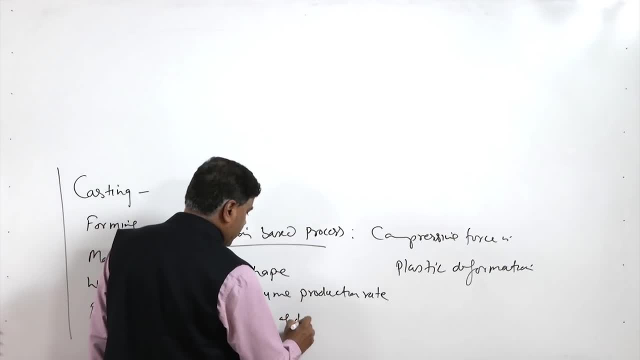 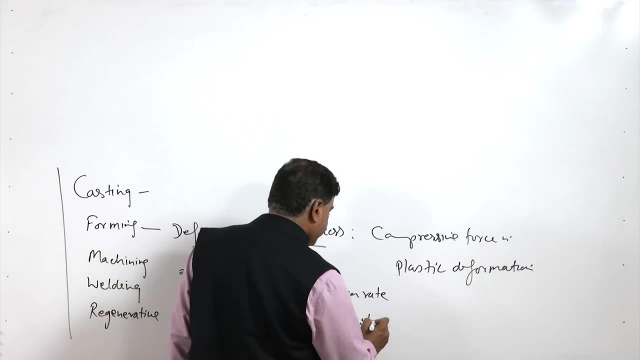 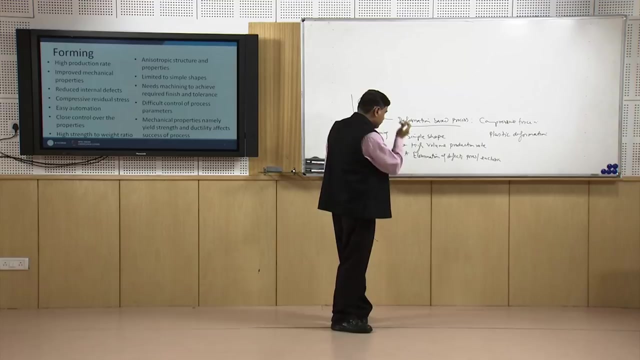 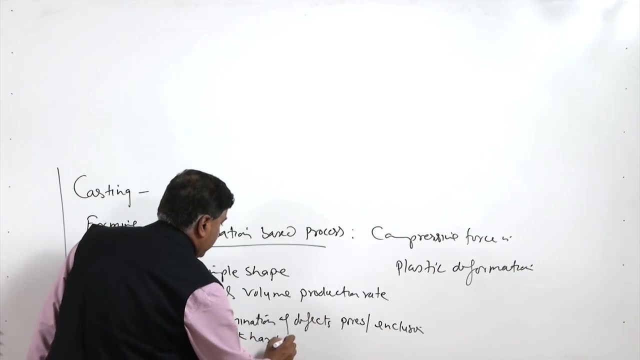 This is the material. So elimination of the defects, like pores or like inclusions are also broken down. So these are, these are made to be discontinued under the deformation forces, under the plastic deformation. So this is the process And at the same time this results in the plastic deformation causes the work hardening. 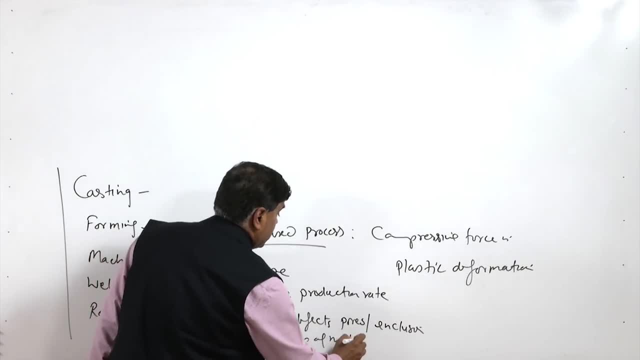 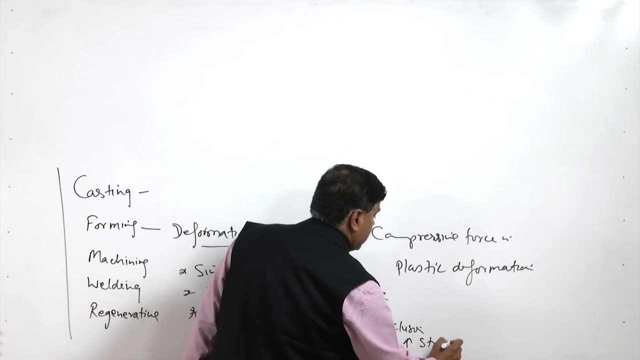 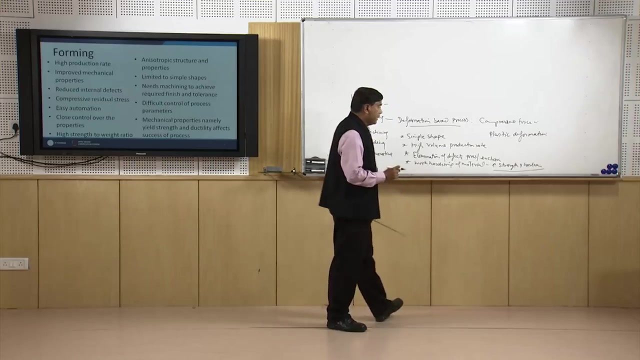 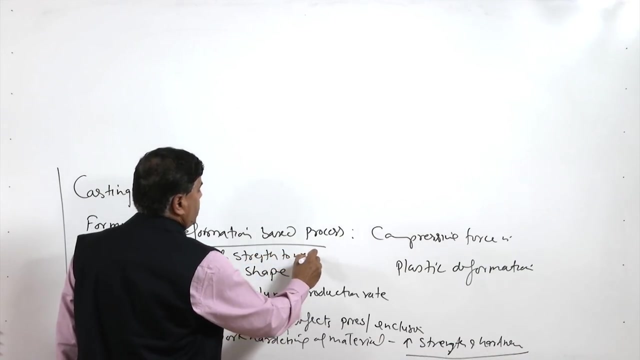 of the material. So work hardening leads to the increased strength and the hardness of the material. So, basically, property enhancement takes place in the products which are made by the deformation-based processes, and this in turn also leads to the high strength to weight ratio. 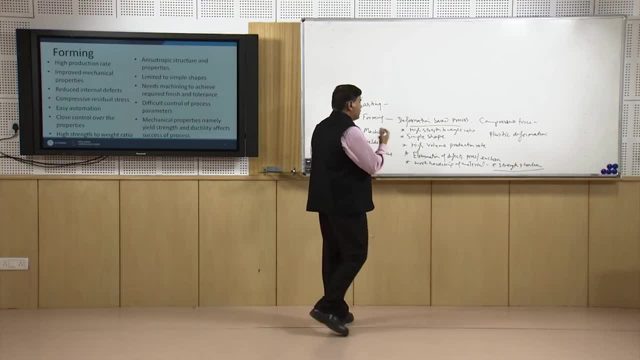 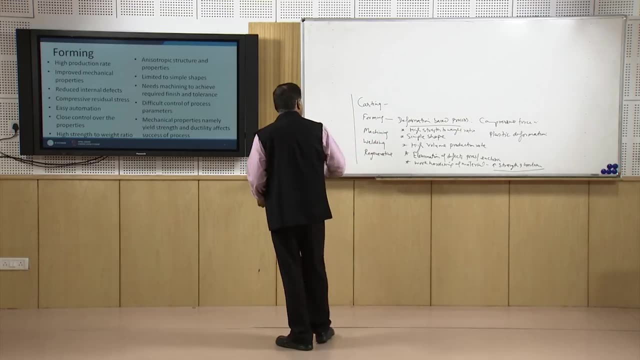 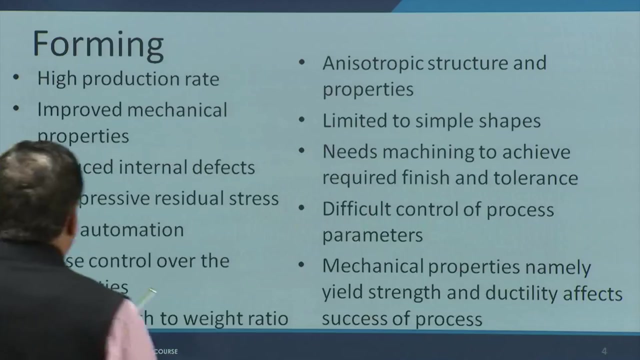 This also helps to increase the achieve the high strength to weight ratio, And these features are therefore exploited in making number of the components for automotive sector. So if we see here the advantages, the forming processes offer: high volume production rate. improved mechanical properties due to the work hardening associated with the deformation. 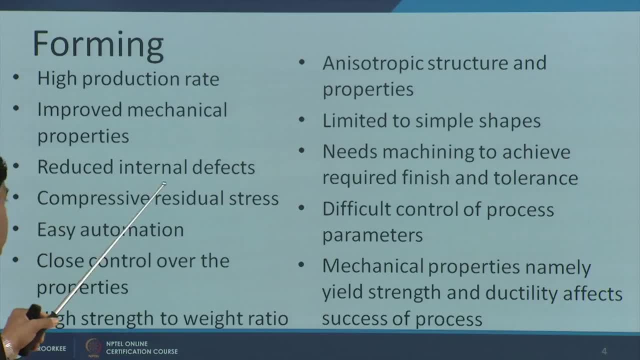 based processes in forming and the internal discontinuities and defects are closed under the effect of the deformation and therefore reduce the internal defects and the compressive residual stresses. Another advantage is the development of the compressive residual stresses. Another advantage is the development of the compressive residual stresses. Since in this process, whenever the deformation takes place by processes like the rolling or the control rolling, here the surface layer deformation is more as compared to the core region and this in turn leads to the presence of the compressive residual stresses, And these compressive residual stresses actually increase the strength of the material. This compressive residual stresses actually increase the capacity to take up the stresses. These compressive residual stresses are considered to be favourable due to the two reasons: one, they increase the tensile load carrying capacity of the product being made capacity and they also improve the fatigue life of the product. 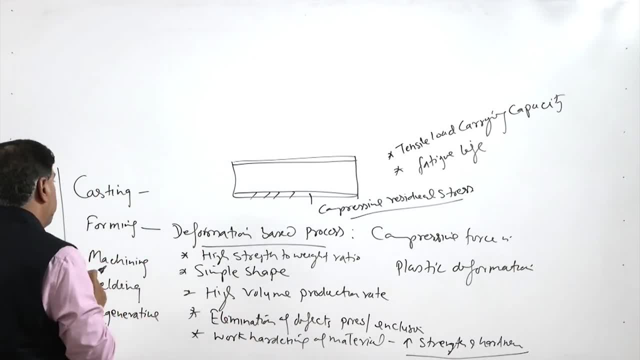 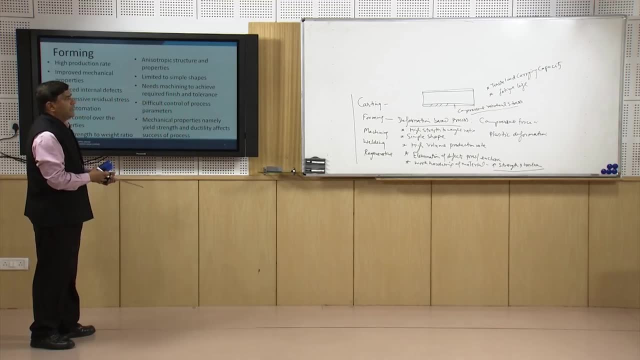 So, because of these two reasons, the component made by the forming process, deformation based process- they will be leading to the improved fatigue life and increase the tensile load carrying capacity and that is considered to be favorable, which in turn helps to make the product by the forming processes of the lighter in weight because of the high strength weight. 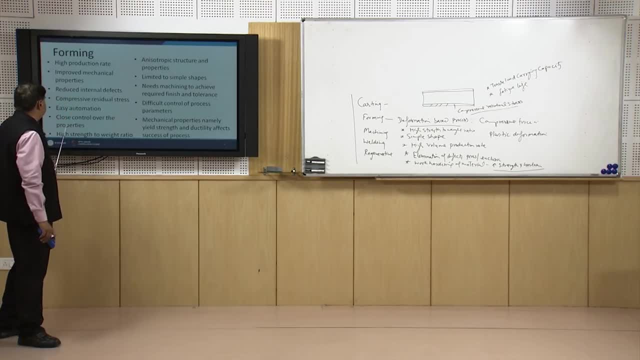 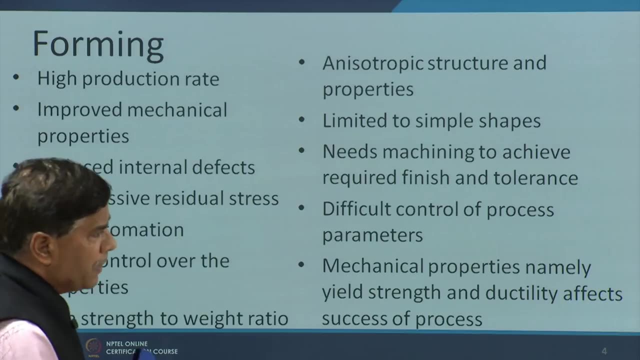 to weight ratio and increased load carrying capacity. Easy automation in these processes and close control over the properties is achieved because we can regulate the extent of the deformation followed by. we can adjust the extent of deformation that we want in each step. thereafter we can use the post forming heat treatment process. 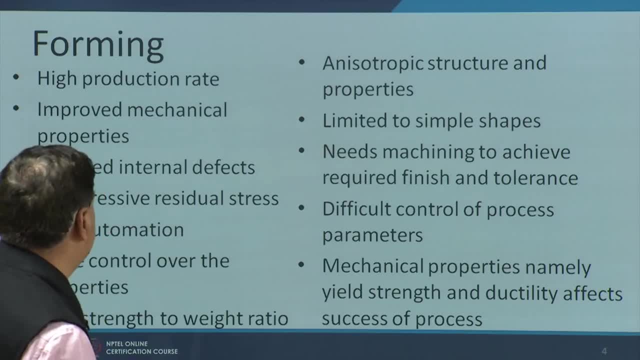 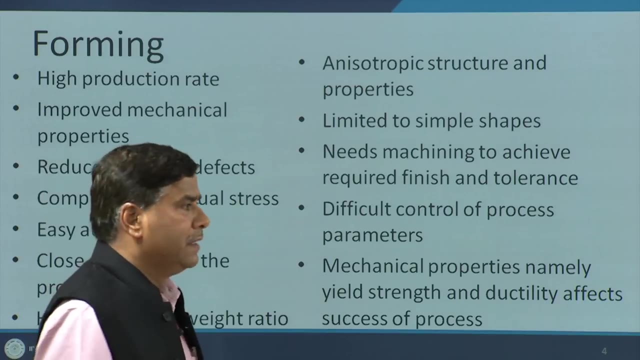 to adjust the structure and properties as per requirement, So the control over the properties is very good. At the same time, high strength to weight ratio is achieved because this process, through work hardening, helps to achieve the higher strength for the same mass of the metal and therefore 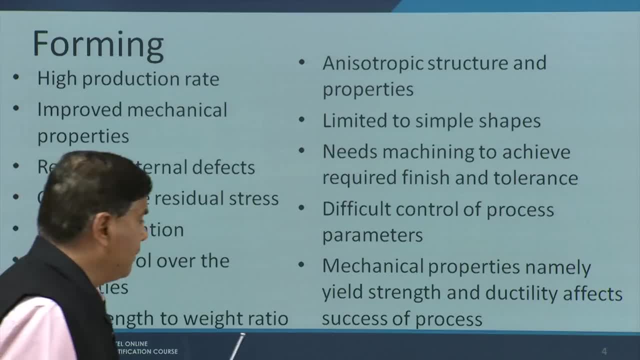 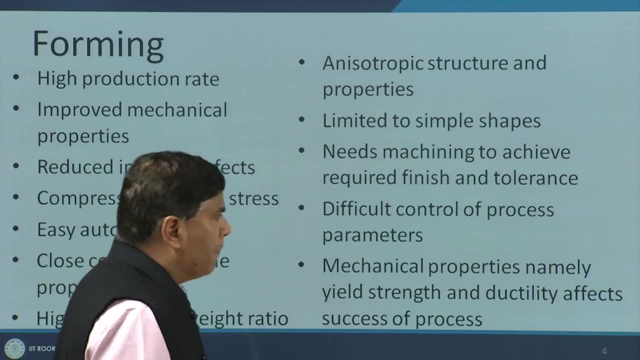 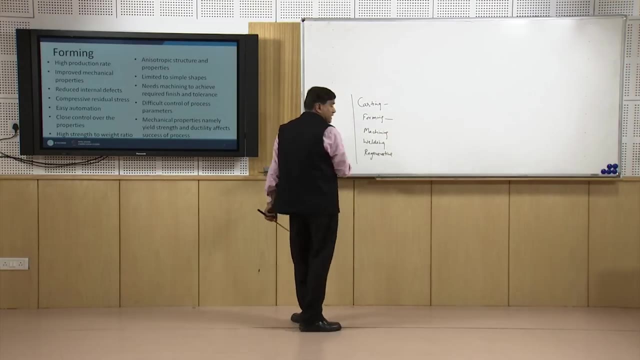 strength to weight ratio, which is achieved by the components made using the forming processes or deformation based process. that becomes quite good, and but there are certain other issues and the limitations related with the forming processes. So these are. So these limitations of the forming processes include, like anisotropic structure and properties. 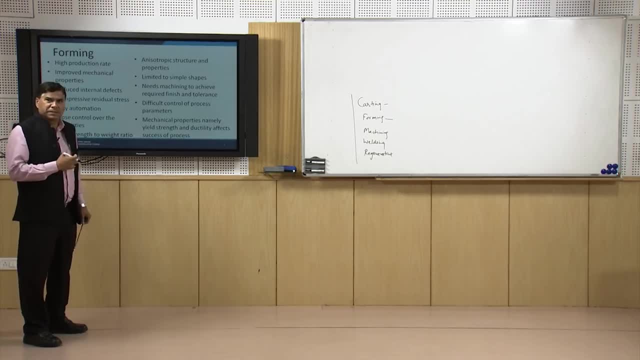 limited to the simpler shapes, because the deformation process really cannot help to achieve very complex shape and very high aspect ratio. sections cannot be made with the complex geometrical features and therefore post machining, post forming machining operations or secondary processing is needed To achieve the desired size and the shape, as well as features, and therefore it needs. 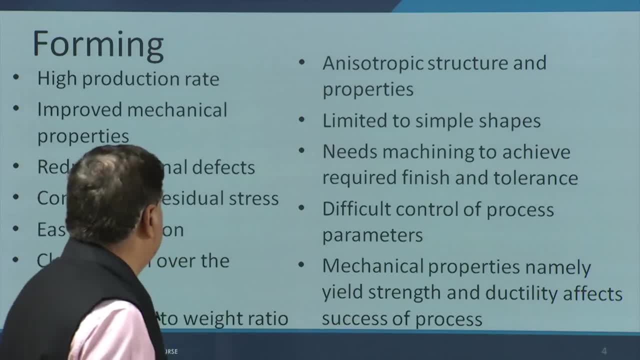 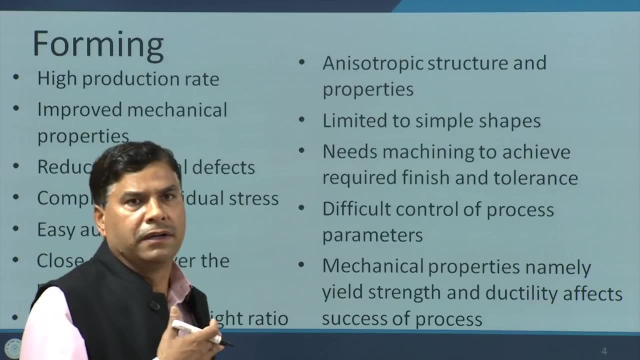 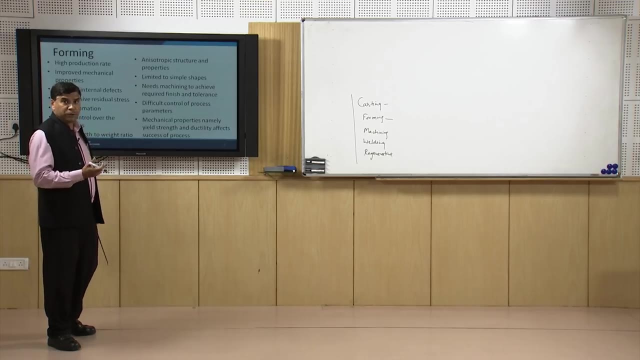 machining to achieve the required finish and the tolerance. The finish and tolerance which is achieved with this process is also not that good because, especially when the hot forming based processes like hot rolling cold and hot forming hot forging is used during the processing, material will be expanding at high temperature. 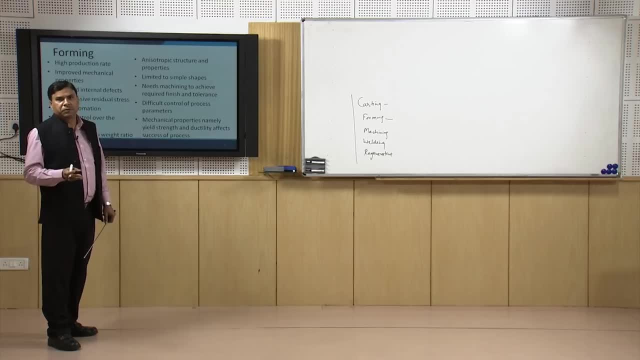 So this process is also not that good. And then if, when it cools down, the shrinkage takes place. So the this changing dimensions of the component due to the heating and subsequent killing, cleaning in case of the hot forming processes especially makes the control over the dimensions. 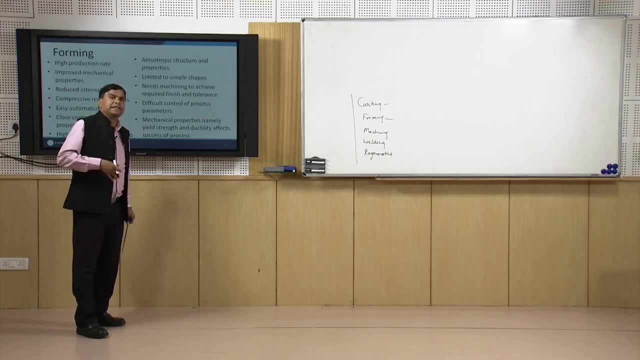 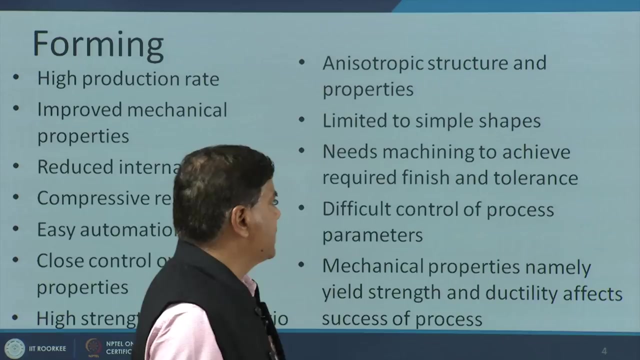 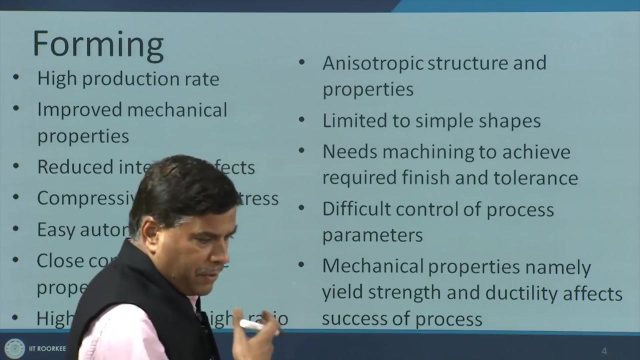 difficult and especially at the same time, increase in temperature also leads to the increased oxidation tendency of the metal and which reduces the surface roughness of the metal. Therefore, the machining is needed so that the required finish and the tolerance can be achieved. Difficult control of the process parameter, since the process is deformation based. so 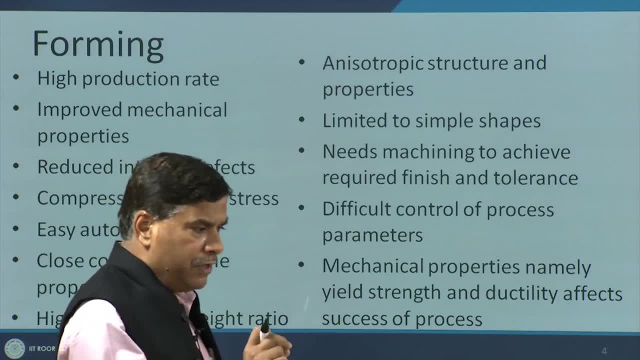 we need to control the temperature of the metal which is being deformed, we need to control the rate at which it is being deformed, and inappropriate control over the temperature, as well as the rate of, as well as the rate of deformation will lead to the development. 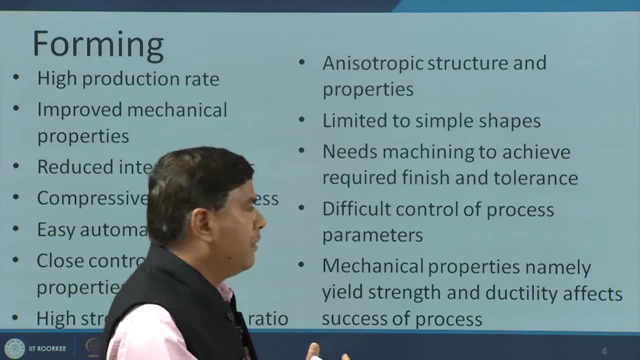 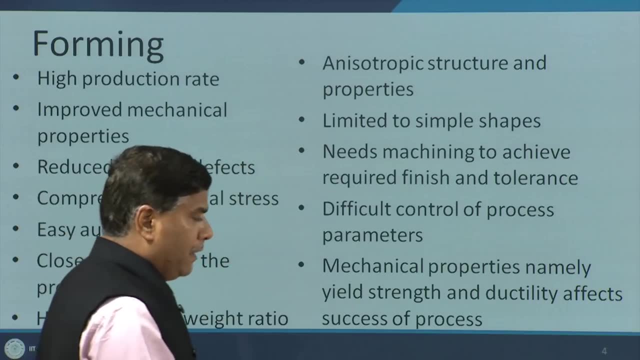 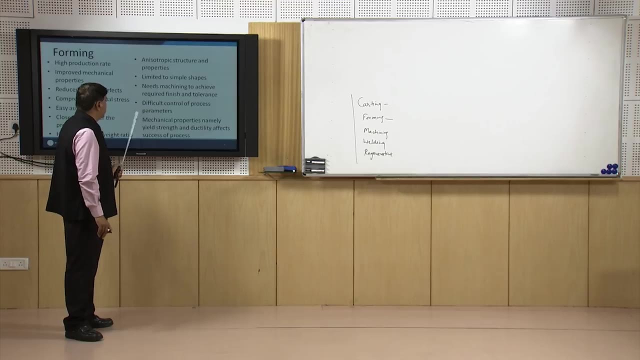 of the surface defects on to the surface of the component which is being made by the forming process and which will lead to the simply rejection or the product with the undesirable characteristics and the properties. Another important point related to the limitation is that the mechanical properties, namely yield, 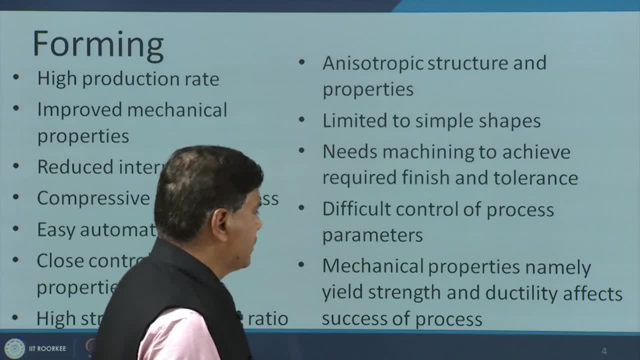 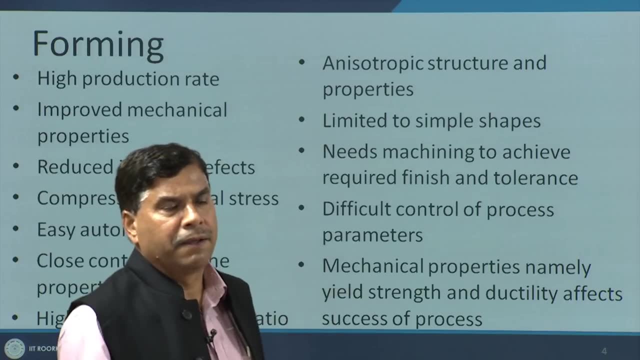 strength and ductility affects the success of the process, and normally, whenever work hardening takes place, The strength and hardness increases, but at the same time the ductility of the work hardened component comes down, so the products which are made using the forming process may be. 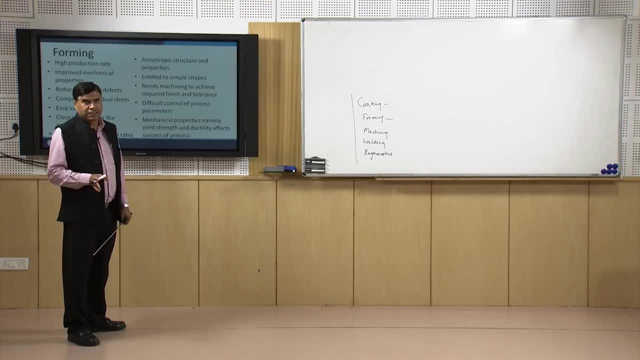 experiencing the localized loss of the ductility as well as toughness. So we need to be very careful. if the application needs, if application of the component made by the forming processes need the toughness as well as the ductility, then in those cases we need to be careful. 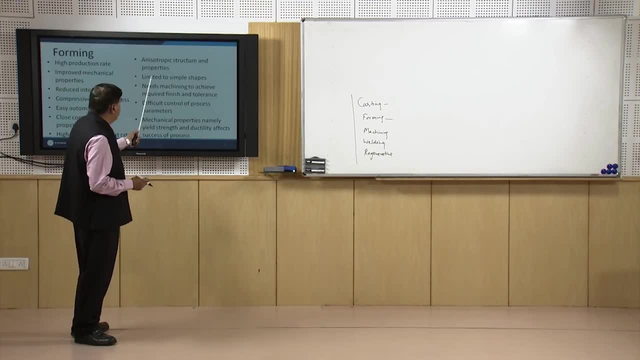 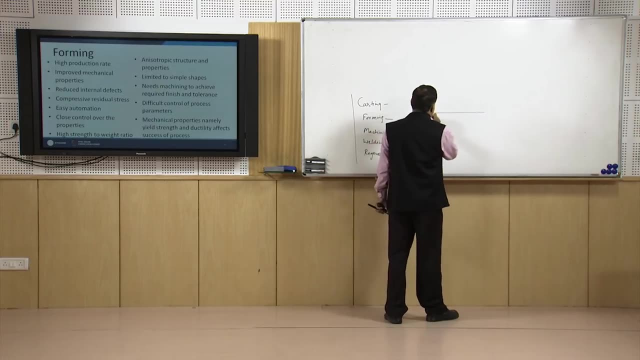 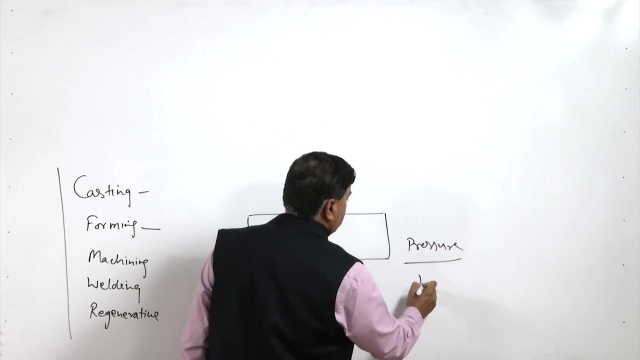 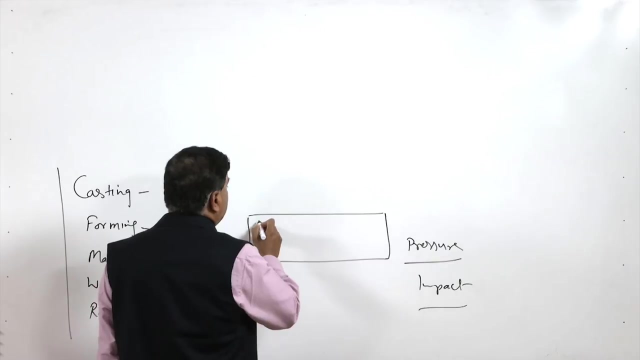 To avoid any premature failure, I will explain little bit more the anisotropic structure and the properties of the formed component. We know that in the deformation we apply, either we apply pressure for causing the deformation or we apply impact. So in case of the pressure and in case of the impact, in case of the impact, the deformation. 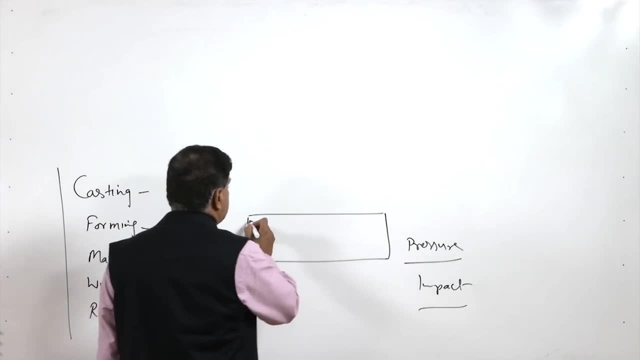 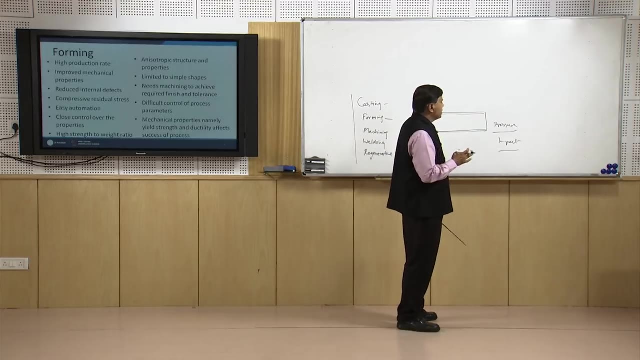 is not uniform throughout the section. Like the surface, layers will be deformed, So it is forming more as compared to the inner core material, while it is expected that deformation in case of the, in those cases where pressure is applied, is by a large uniform. 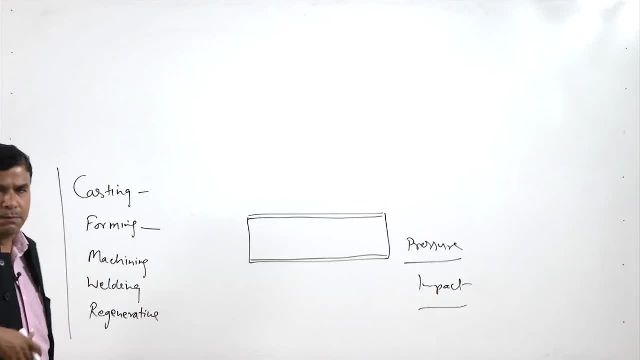 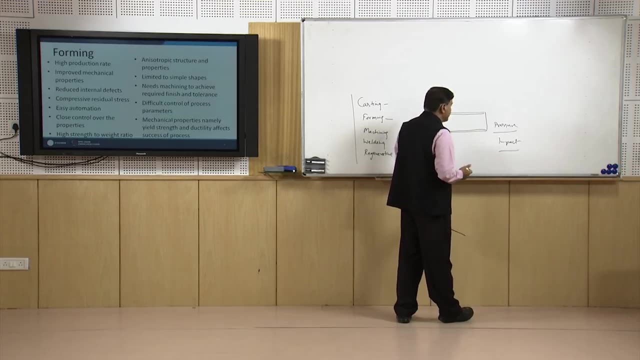 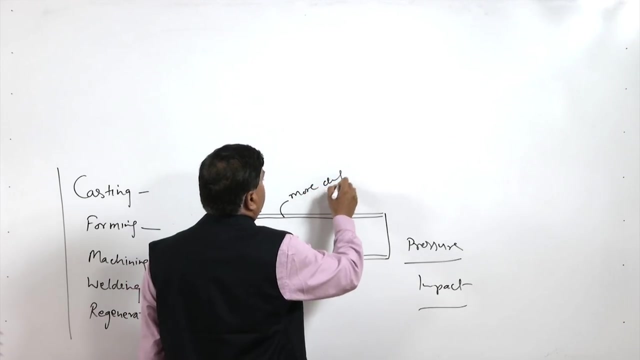 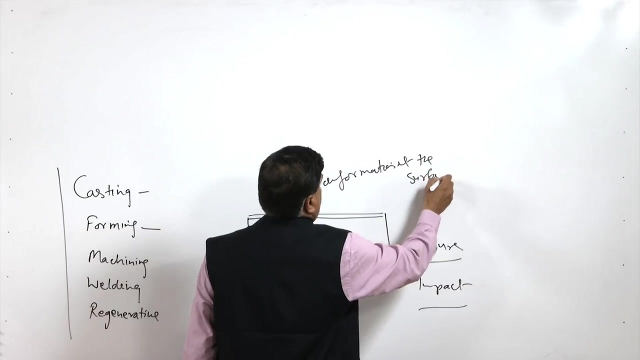 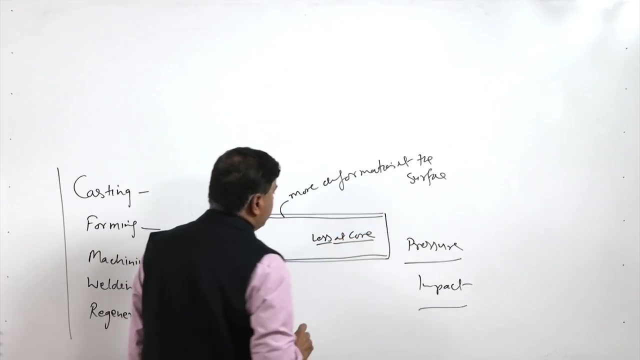 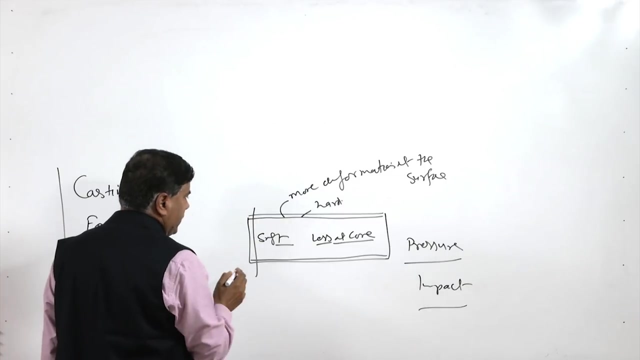 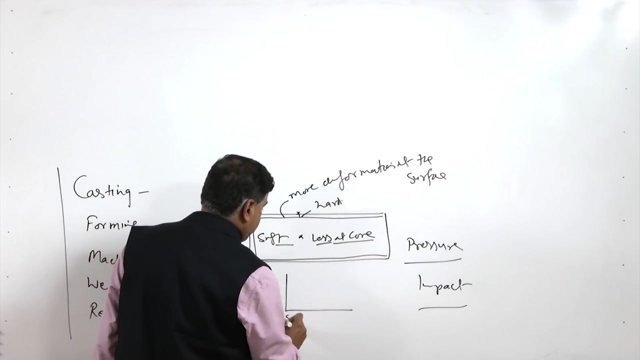 but is still the deformation is more experienced at the surface as compared to the inner core material of the component which is being deformed to get the desired size and shape. and because of this differential deformation, more deformation If you measure the properties from the surface to the depth, so from the surface to the core. 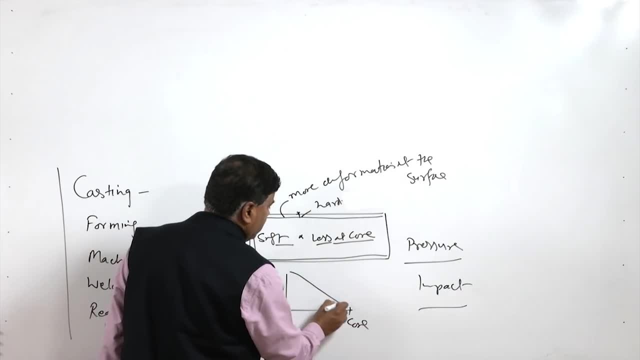 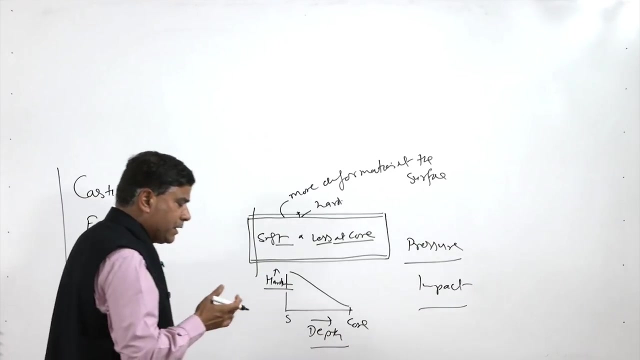 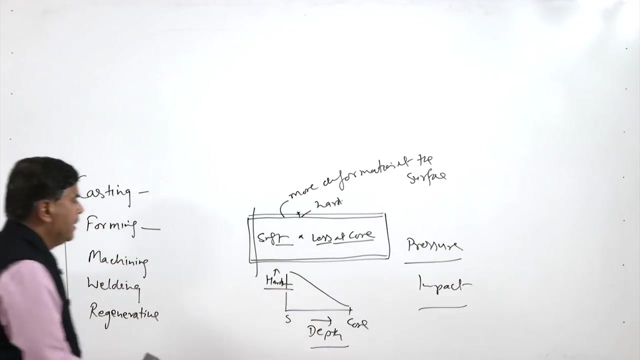 of the material, we may find that there is continuous drop in the hardness and strength of the material with the increasing depth from the surface. So with this kind of the trend, the differential property variation is attributed to the difference in the work hardening. So the material after deformation is less, and this is theней way of determining the. 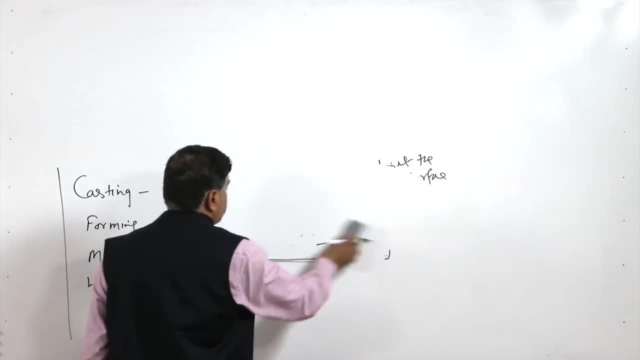 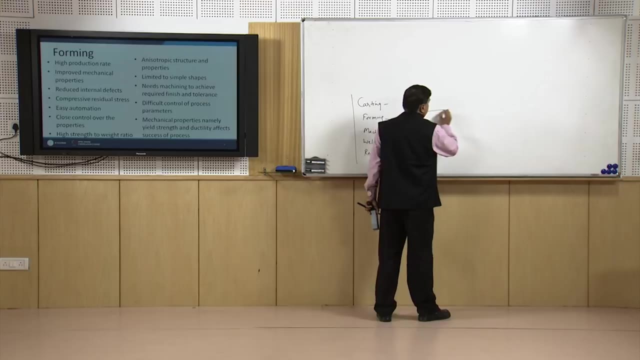 force because, as we said, the force is not always constant in the process. The very most important thing which is observed is, during the deformation based processes, material is forced to flow in a particular direction, which is called longitudinal direction, and that, due to the application of the force, material flows in one particular direction. 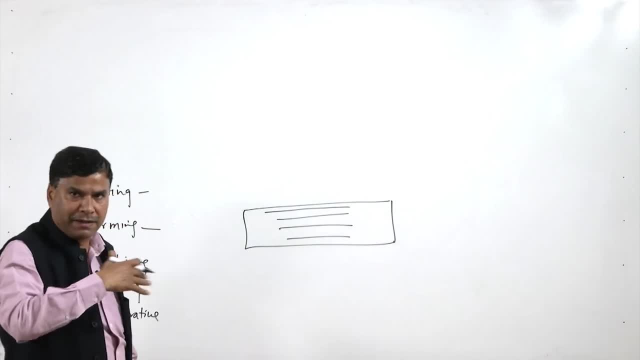 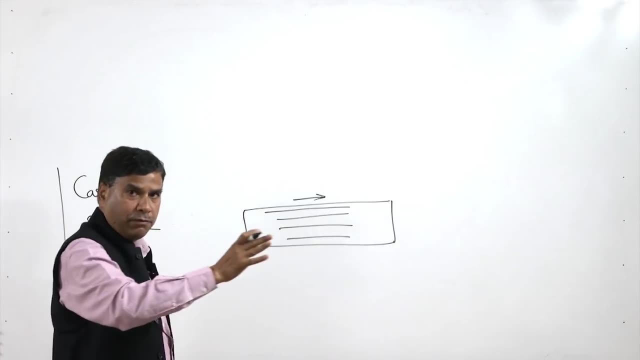 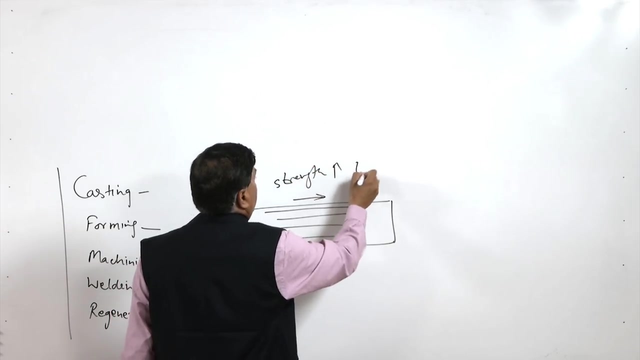 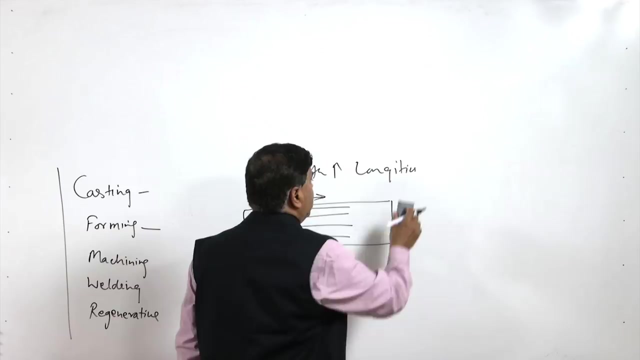 So the direction in which material flows, we find much better strength as compared to the direction perpendicular to that, So longitudinal direction, which the grains will be flowing. the strength is found to be much better as compared to, the strength is high in longitudinal direction, or the direction in which the flow of the 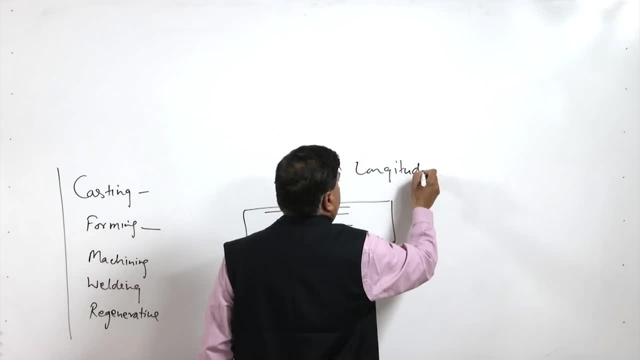 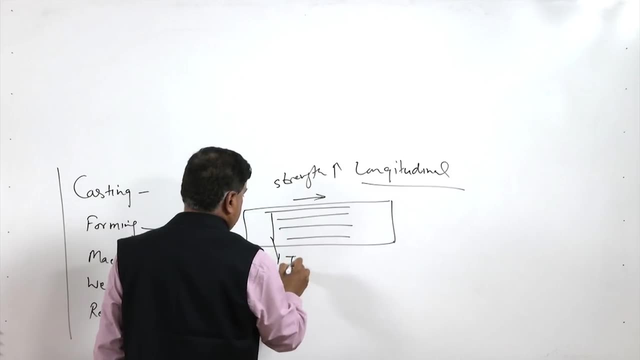 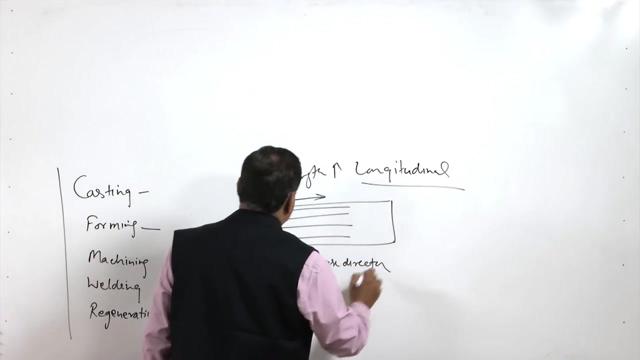 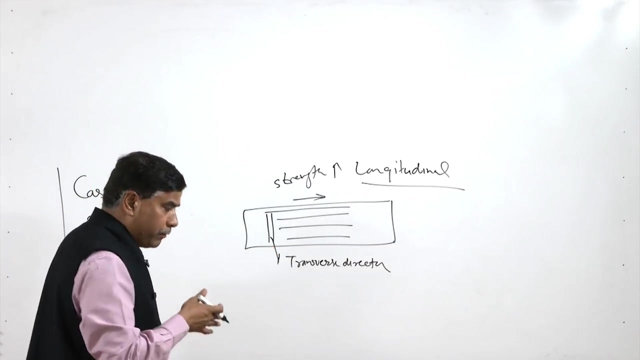 grains take place during the deformation: longitudinal and the transverse. transverse direction is this. So the properties in the transverse direction means the direction perpendicular to the flow of the grains. the perpendicular, the direction in which the grains have flown under the effect. 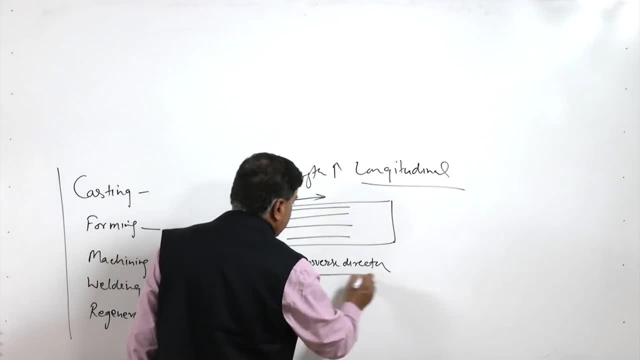 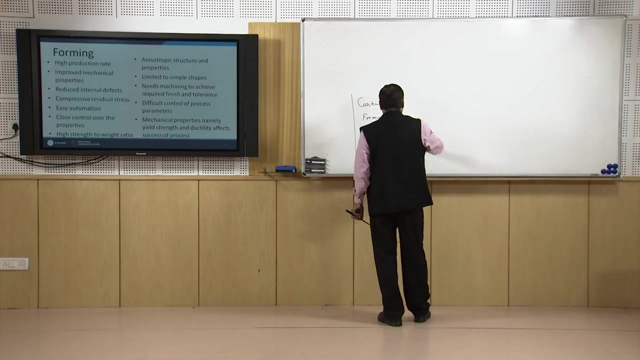 of the external forces. that direction is the transverse direction and in that direction the strength and strength is found to be lower than the longitudinal direction. So this is another aspect. so, while designing the manufacturing process or while deciding the direction in which the flow is to be achieved, we need to consider the way by which the material 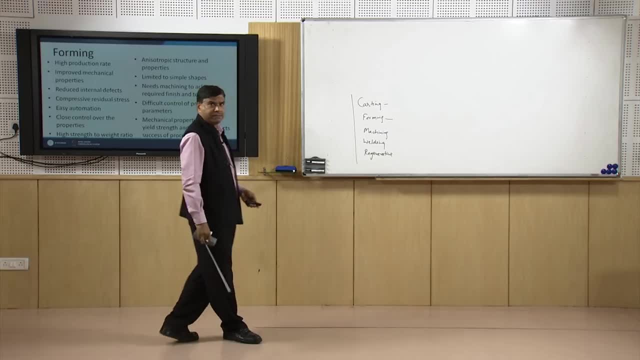 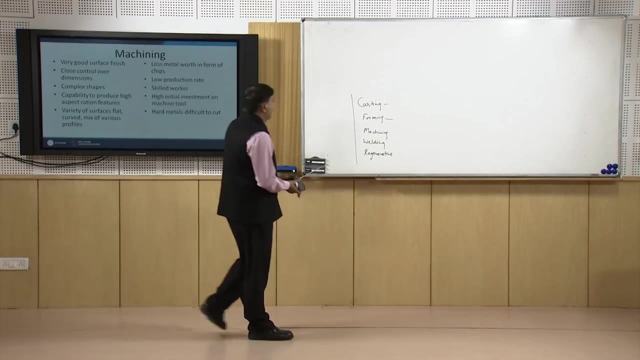 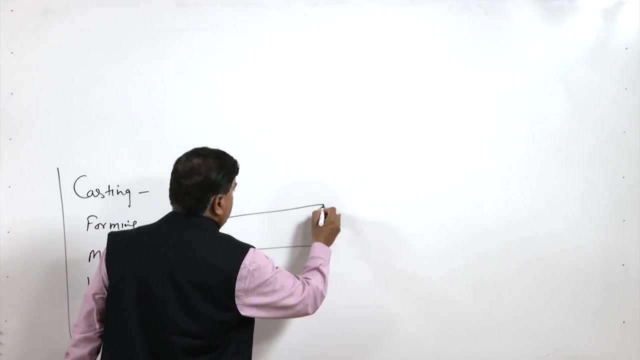 will be subjected during the service. Coming to the another machining process, another manufacturing process is the machining one. We know that in case of the machining, We take the stock material, like this and, using the suitable cutting tool, the unwanted material or unwanted extra material, like, say, this is the unwanted, this is the shape which is to 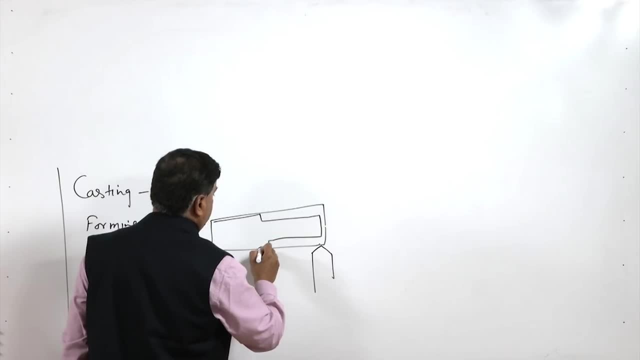 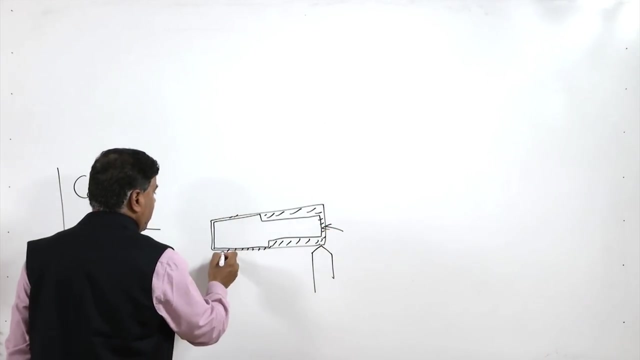 be achieved. so the unwanted extra material will be removed by. so this hatched portion is the portion where from material is to be removed. Say: this is the turning process, This is where facing will be done. this is the turning region and this is the region. 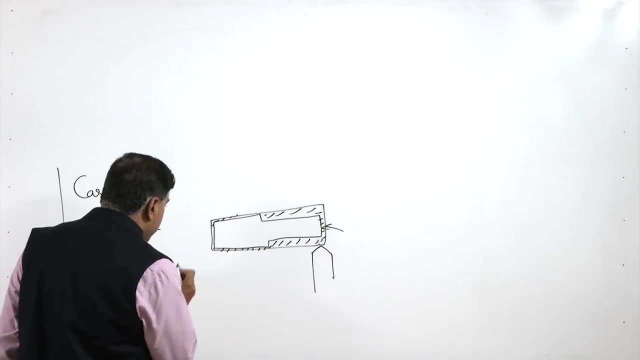 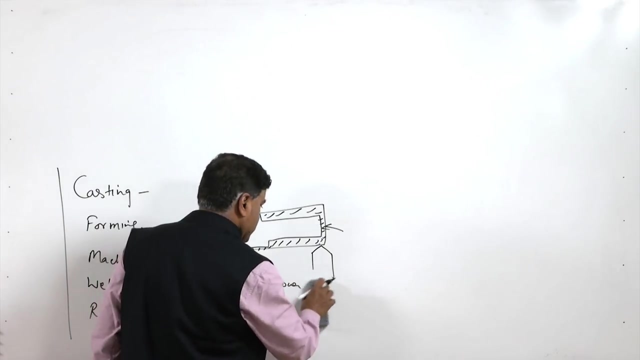 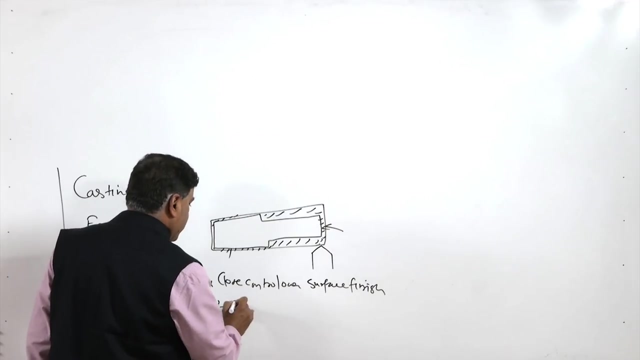 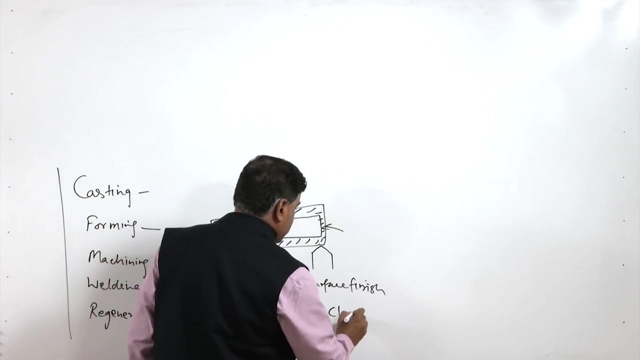 where turning is to be done. So when this is applied, what we get? We get very close control over surface control over the surface finish. This is one, This is the whole- And very close control over the dimensions. So very close tolerance can be maintained using the machining process. 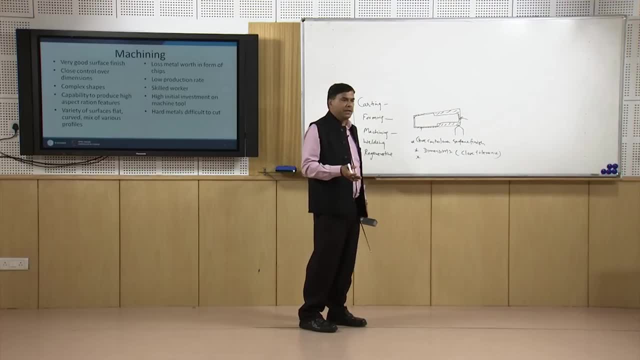 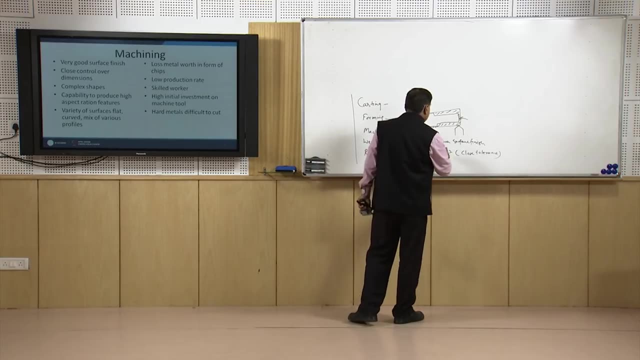 That is another. that is why most of the formed component or the cast component are processed through the machining. So that the desired control over the dimensions, So that the desired control over the dimensions And the machining process, That is another. 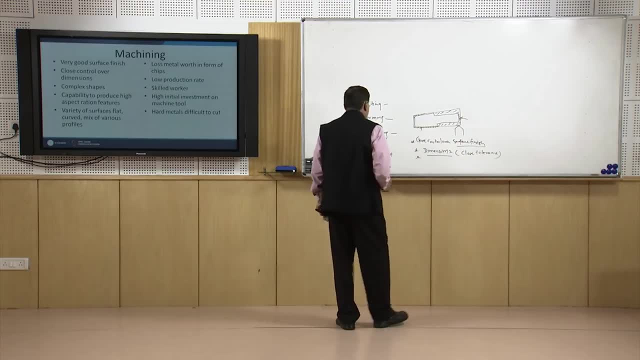 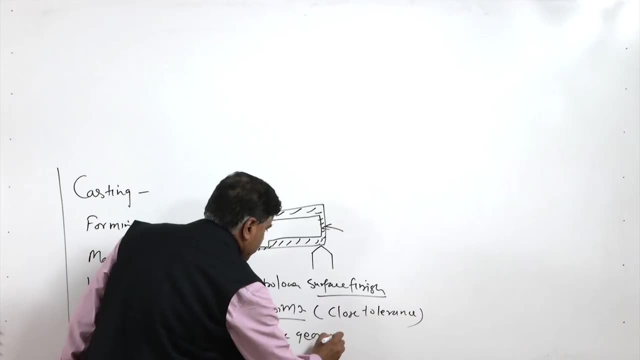 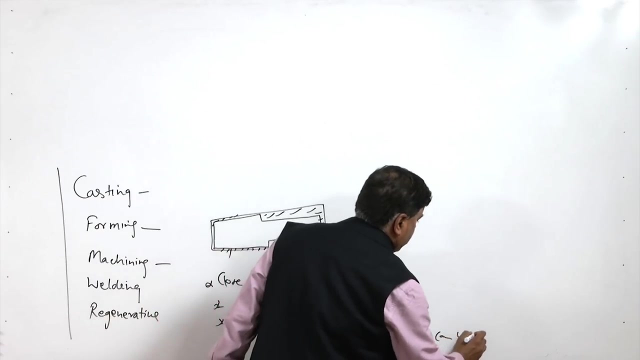 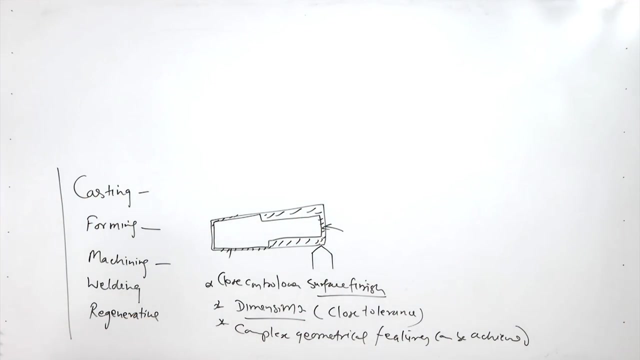 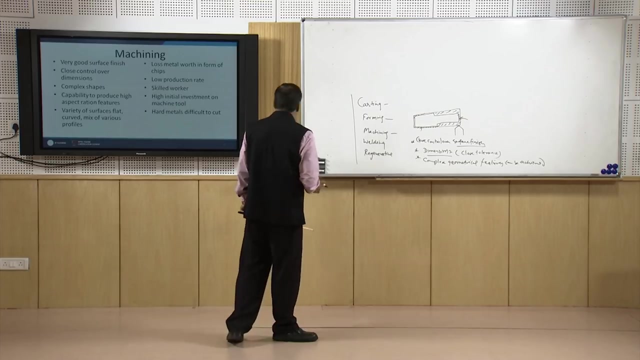 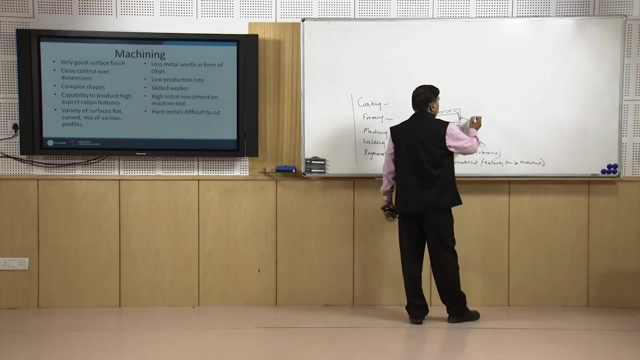 surface finish can be achieved. At the same time, very complex geometrical features can be achieved by machining, which is otherwise not so easy to be made in case of the casting and forming with the such precision as well as the good surface finish. So the complex geometries can be achieved, but the process has the limitation of the 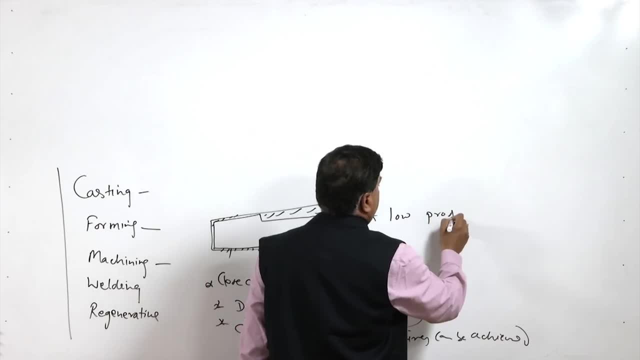 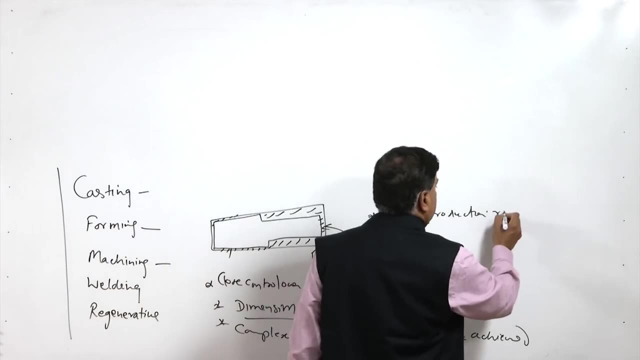 low production rate because the material is removed sequentially, one by one, So it takes long to achieve the desired size and the shape and there is a loss of metal worth material whatever is removed, So metal is lost and cannot be used further for any other useful purpose and therefore 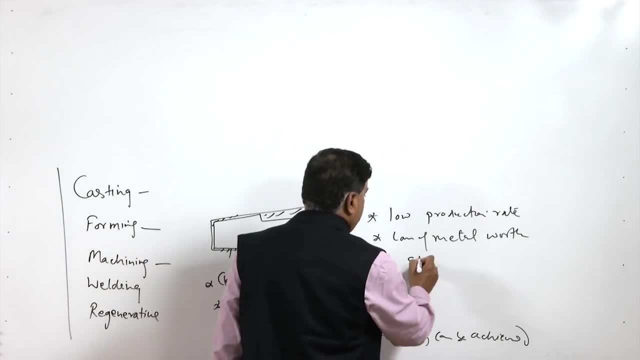 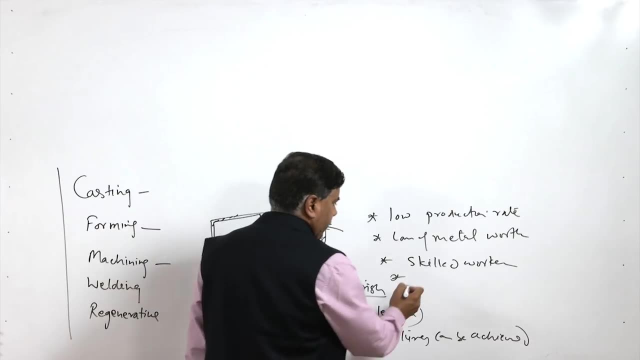 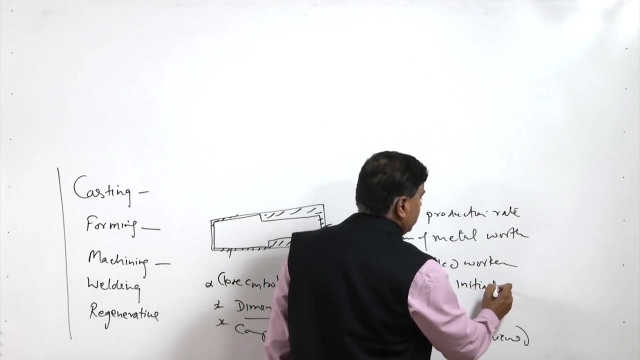 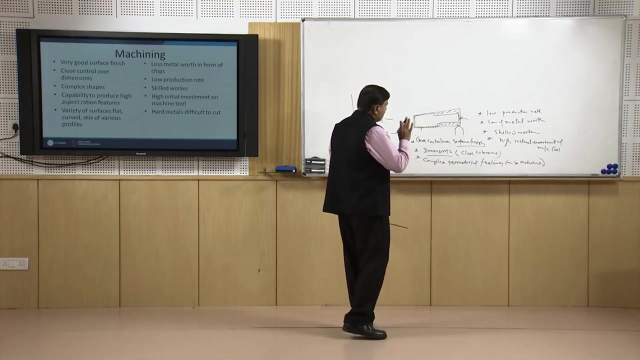 the metal loss takes place, very skilled worker or machinist is needed for the machining purpose and high initial investment on the machine tool is needed- high initial investment on machine tool. So these are some of the limitations. at the same time, we know that to facilitate the machining, 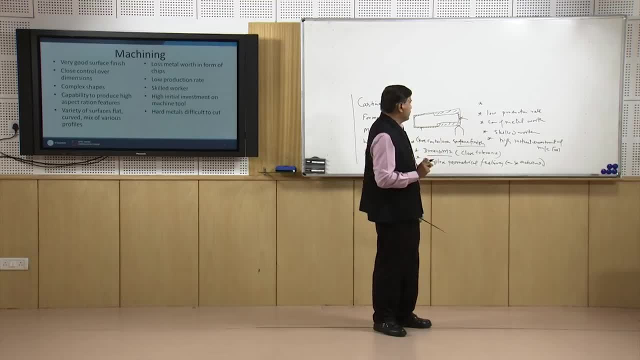 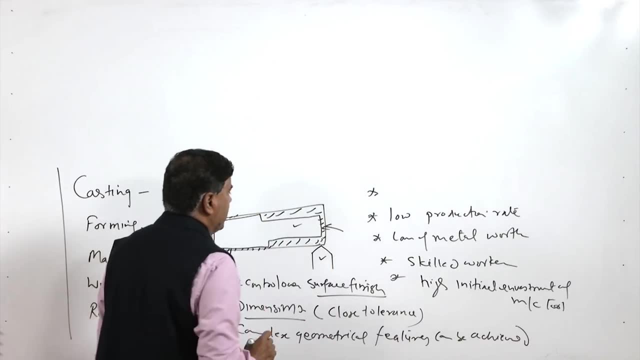 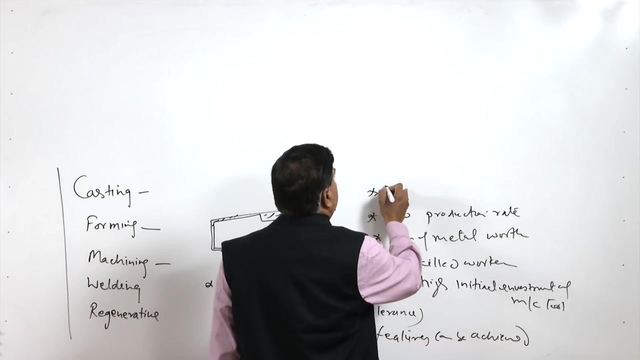 of a material, it is necessary that tool penetrates into the work piece. but that penetration will be possible only if the tool is harder than the work piece. If the work piece itself is harder than the tool, then it will not allow, It will not allow any kind of penetration, and that is why the work piece of high hardness- 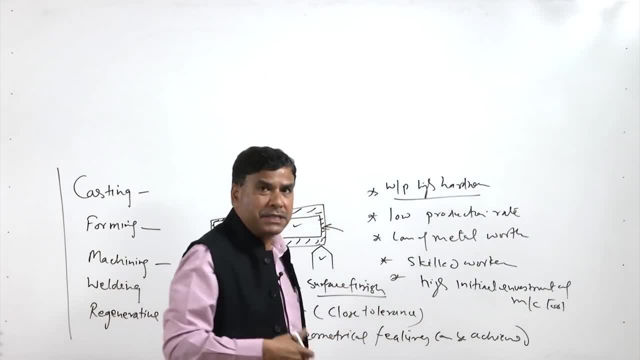 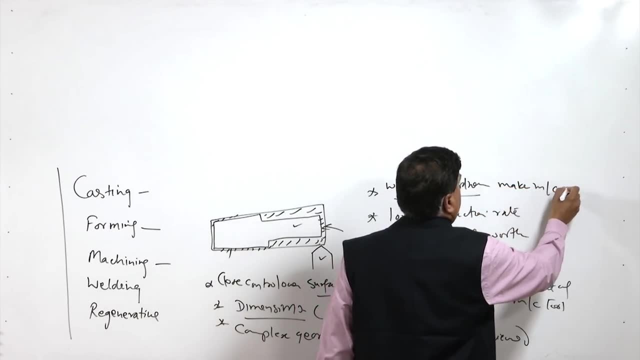 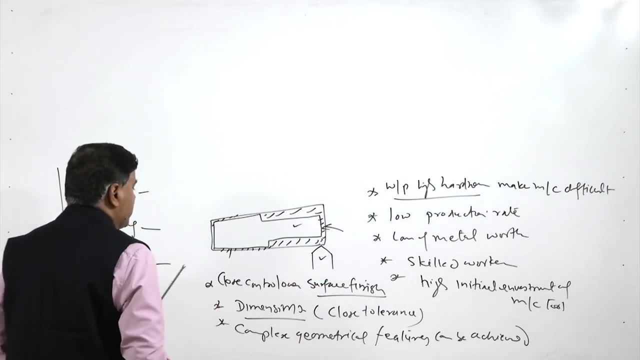 they offer resistance. they make the machining difficult. So high hardness materials make machining difficult by the conventional process. This is another one. so high hard means the materials of the very high hardness cannot be easily processed. So that is the the also one which is of the unique feature for the machining process. 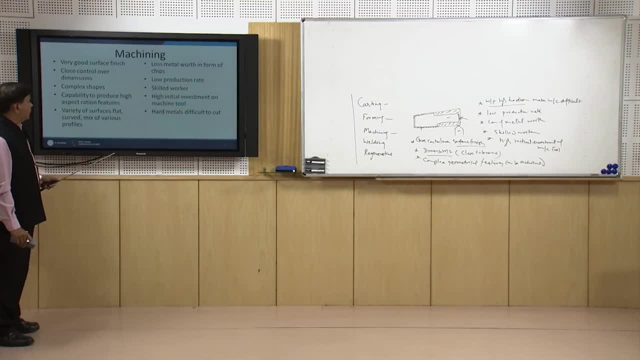 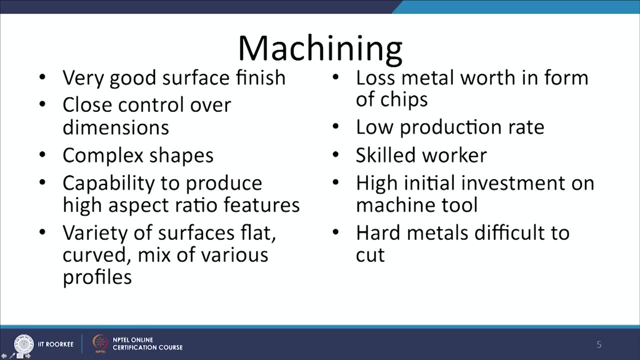 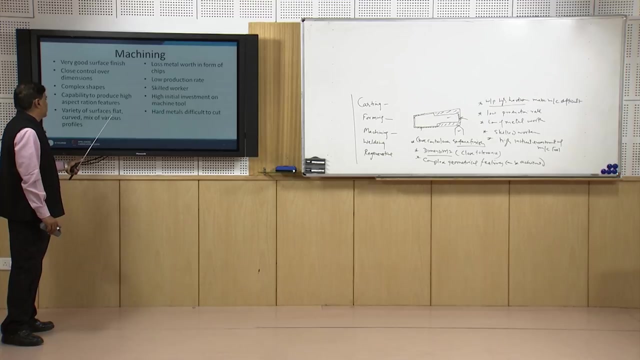 So the advantage side, very good surface finish, very close control over the dimensions and very complex shapes can be produced and it is capable to produce very high aspect ratio features which otherwise cannot be made using the like forming and the casting processes and the variety of surface features, like the flat, curved or mixed of the various profiles. 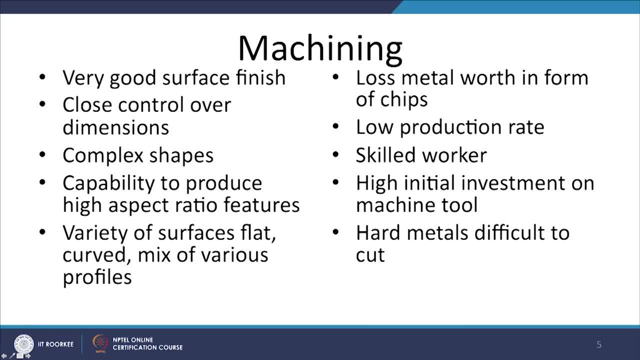 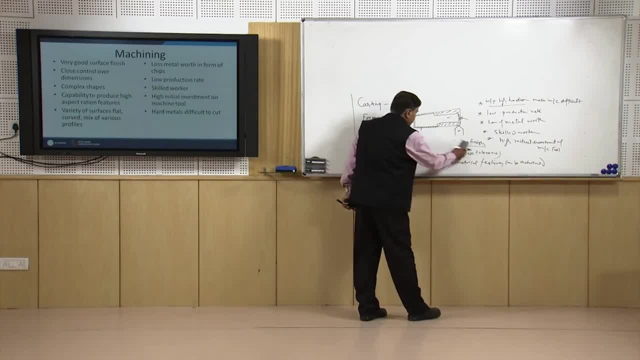 can be easily made. So this is one of the advantages. So the advantage side, very good surface finish, very close control over the dimensions, and So these are the advantages and these are the disadvantages and the limitations associated with the machining processes. Coming to the welding processes: welding, you know the welding or you can say the joining. 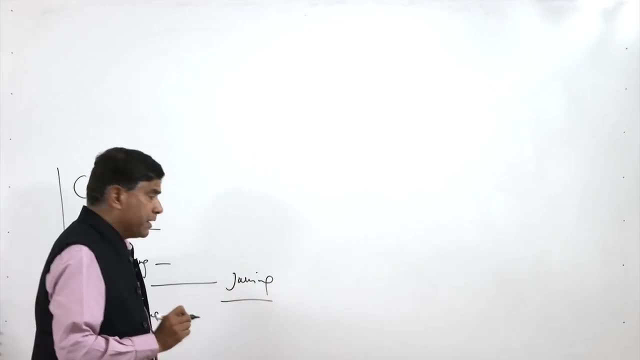 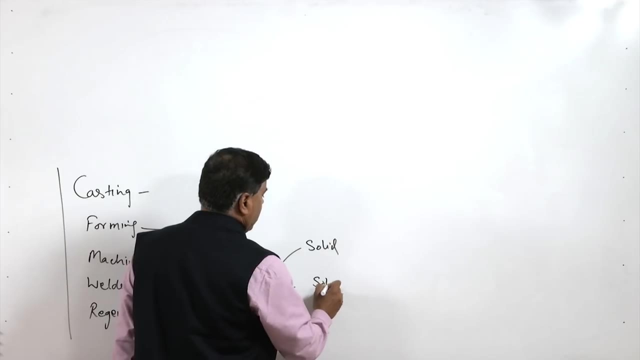 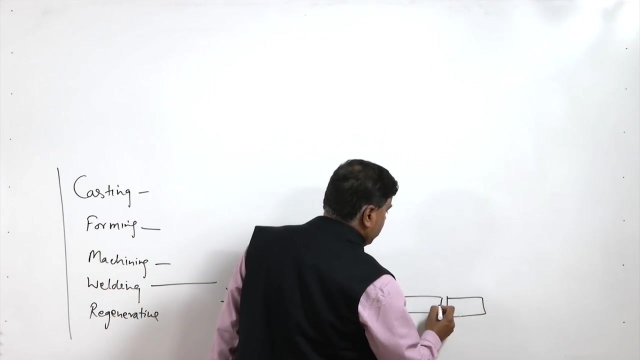 processes. there are three variants in the joining processes, like the solid state joining processes, solid and liquid state joining processes and the liquid state joining processes. So liquid state joining processes, where the components to be joined need to be brought to the molten state with the application of the heat. 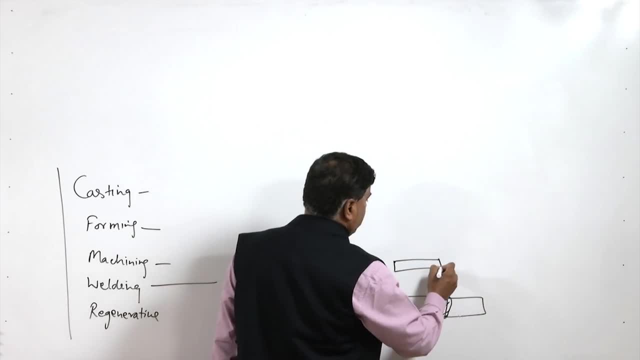 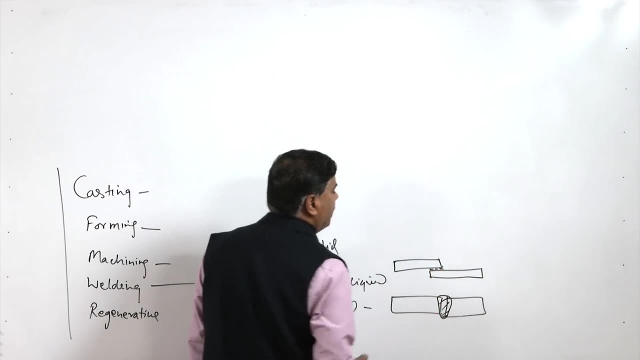 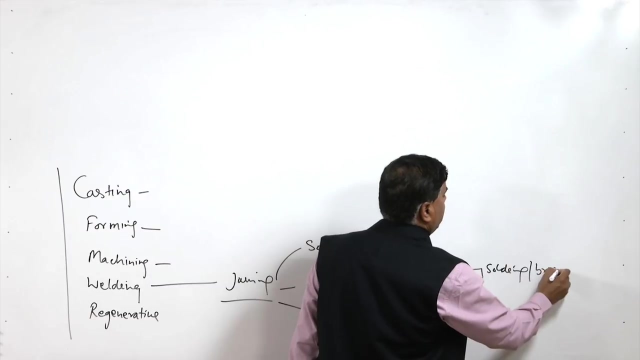 In case of the solid liquid joining processes, what we do? The components to be joined are just heated So that the material, So low melting one material can be filled in. So the processes like shouldering and brazing fall in this category, while in case of the 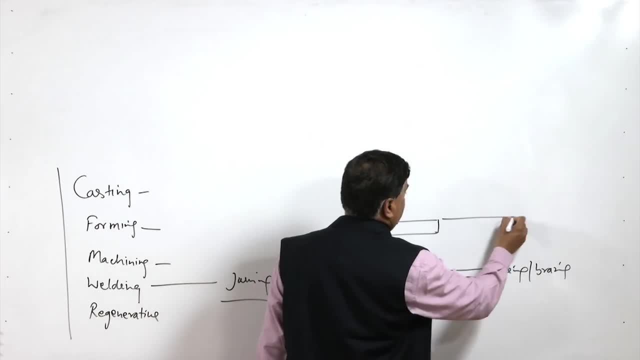 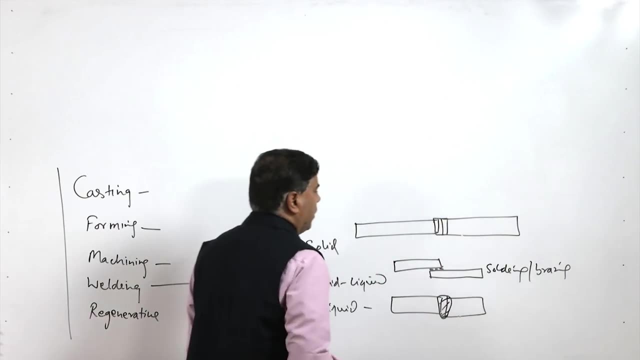 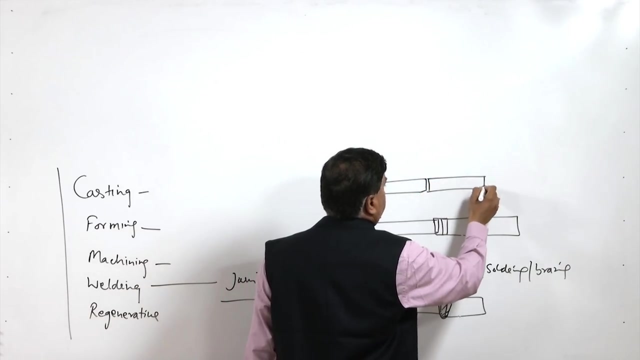 solid state joining processes. the components are maintained in the solid state and application of the force helps to make the to have the metallic continuity as well as, or. we can use the processes like the diffusion, where cleaned, polished surfaces are kept under the pressure at high temperature. 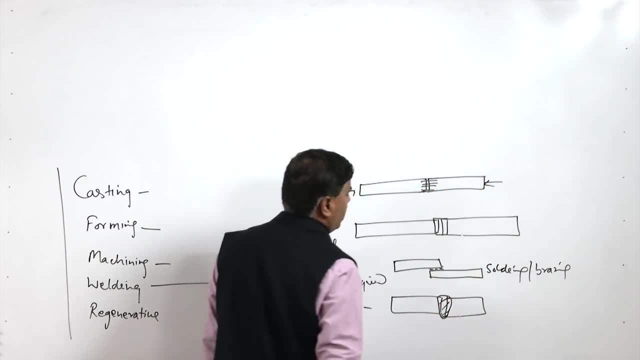 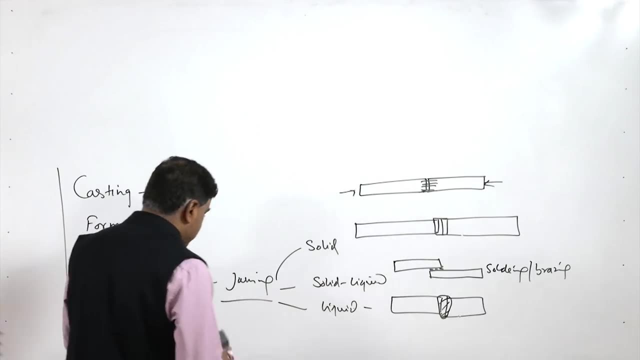 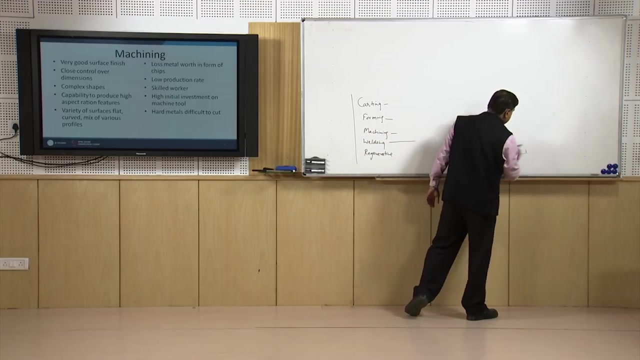 So that the diffusion across the interface takes place to have the metallic continuity. This is about the process. So the range is so wide that it allows very good features to the joining. So if we go by the advantages related with the joining processes, it helps to make very 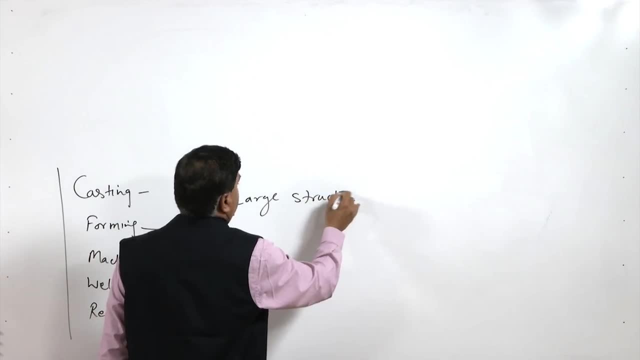 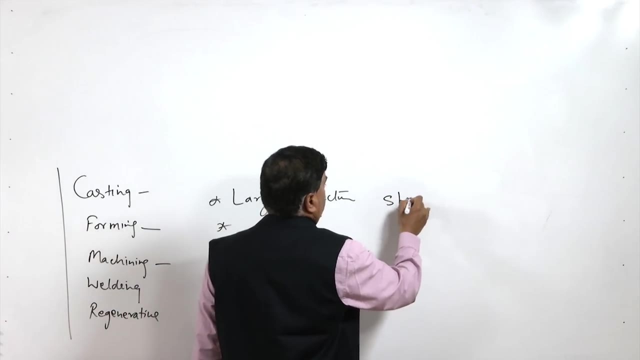 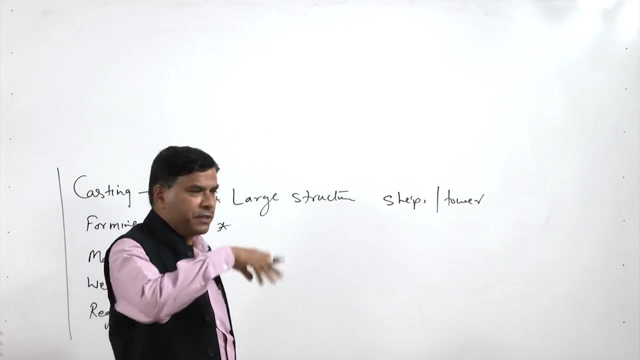 large structures. It allows to develop the large structures. So this is the process, So the production of the large structures like ship, or big towers like Eiffel tower is also one of the example where simpler shapes are joined together to make a big tower. 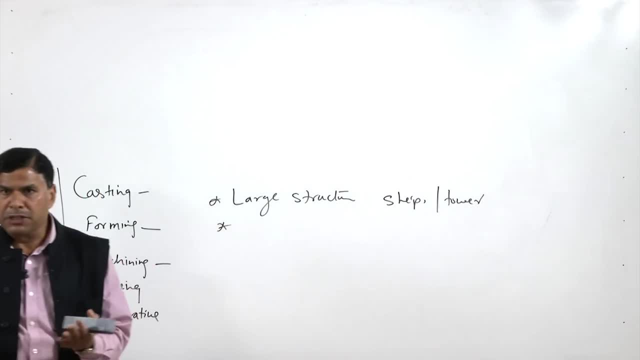 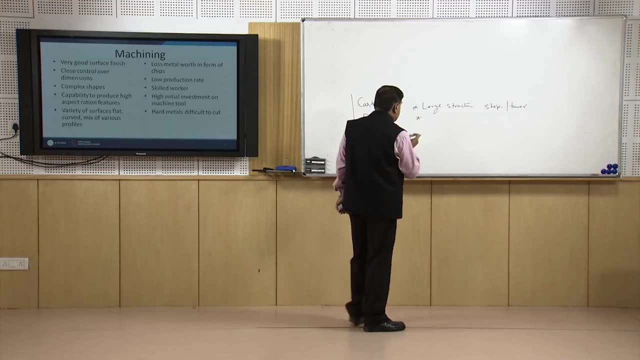 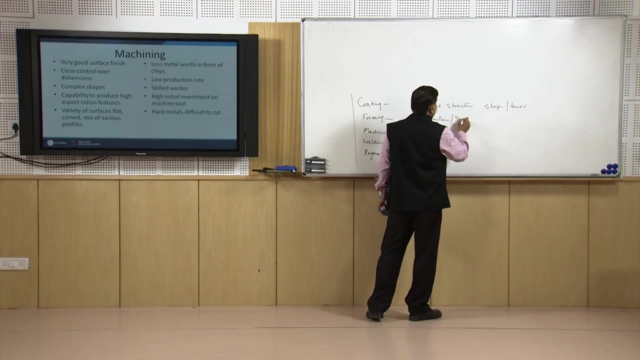 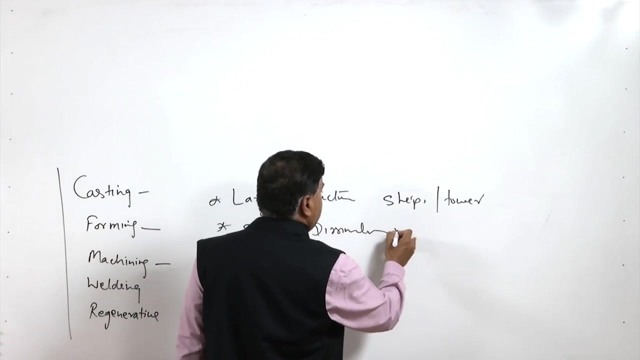 So here what we do for fabrication of the ships: The simpler plates are joined together by welding to achieve the large size structures. Another thing it can make: It can help to develop the joining of the similar and dissimilar. Both similar and the dissimilar. joints can be similar and dissimilar metals can be joined. 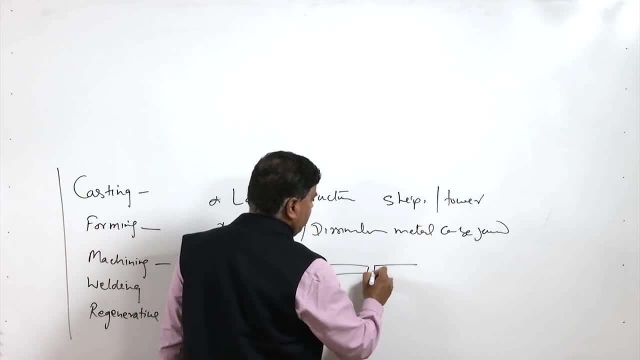 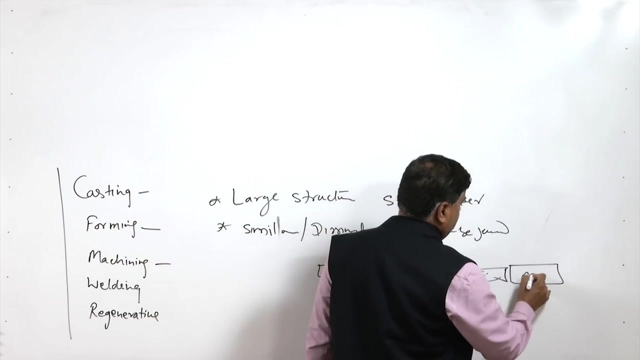 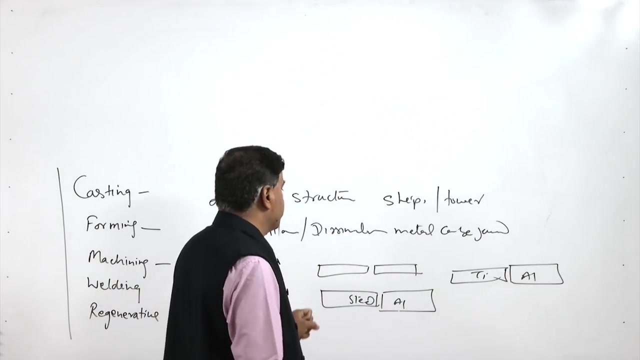 Because there are examples like joining the paper with the metal or joining the like, say, steel with the aluminium, or joining of the titanium with the aluminium. So there are very means. the completely different kind of the metal systems can be joined using the suitable combination of the process, whether it is chemical based, like the adhesives can. 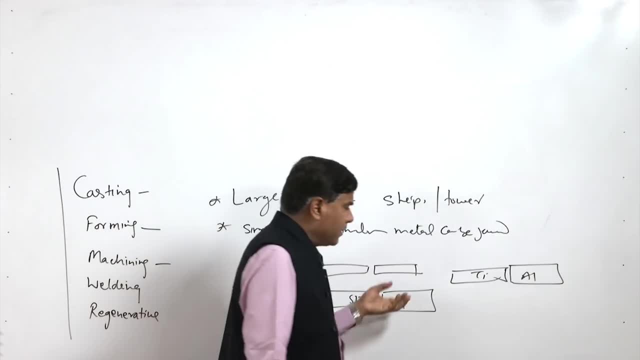 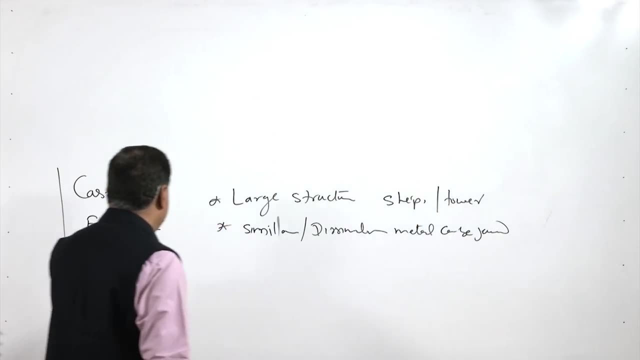 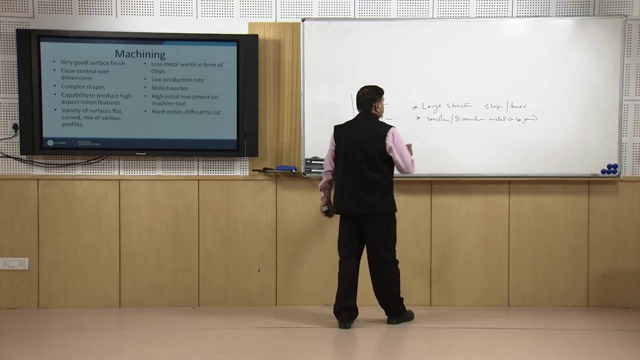 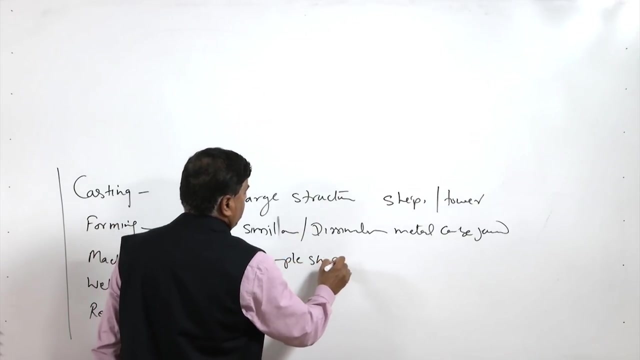 be used, or like solid state joining process, or the solid and liquid state joining process can be used As per the compatibility, The suitable kind of the process. joining process can be selected to have the joint between any two systems, So large structures. so the good feature is that it uses the simple shapes to get the 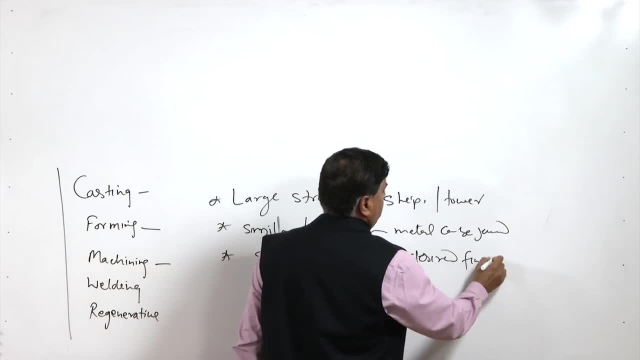 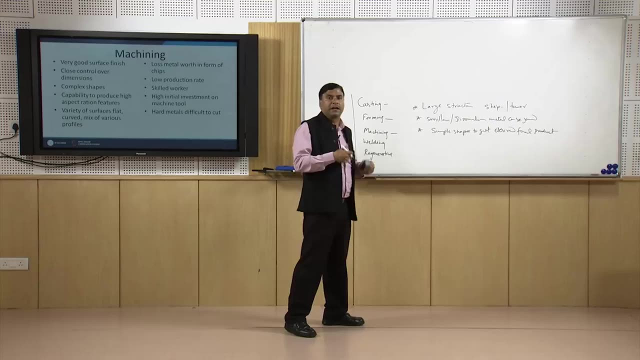 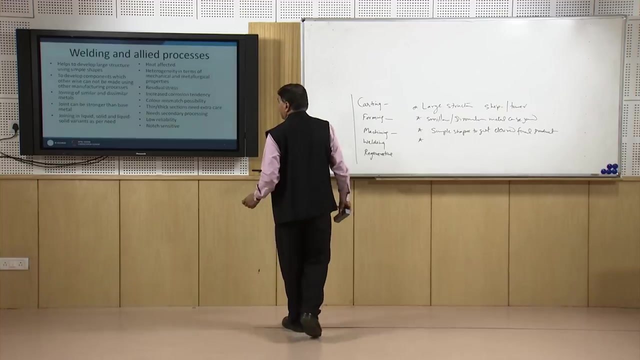 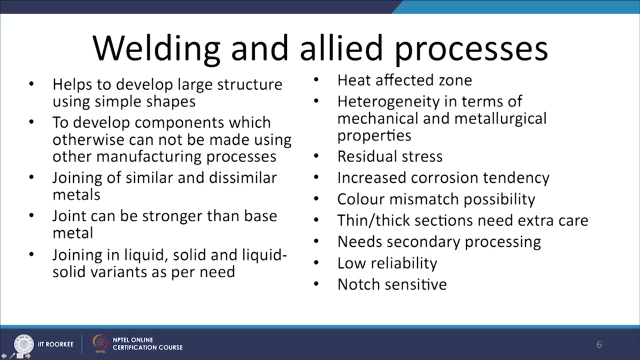 desired final products means this process is good for making those shapes Which cannot be otherwise be realized through the forming or the casting processes, or the machining will be uneconomical. So that is the another side. So, coming to the advantages of the welding and alloyed processes, if you see here it 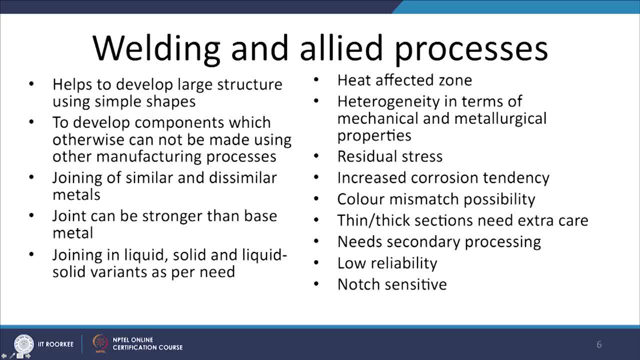 helps to develop the large the welding processes. helps to develop the large structures using simple shapes, Like ships and towers, to develop the components which otherwise cannot be made using the other manufacturing processes. like it, using the simple shapes we can make the components otherwise very easily, more economically otherwise, which will be difficult, using the forming or casting. 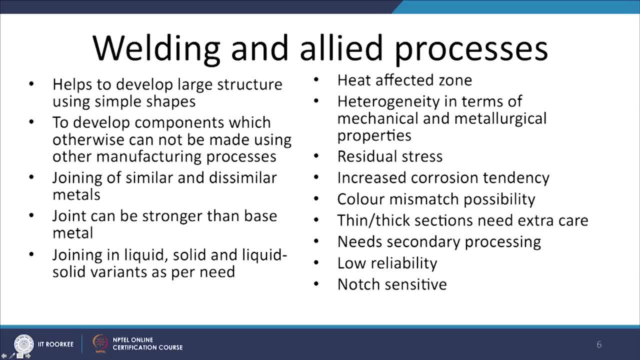 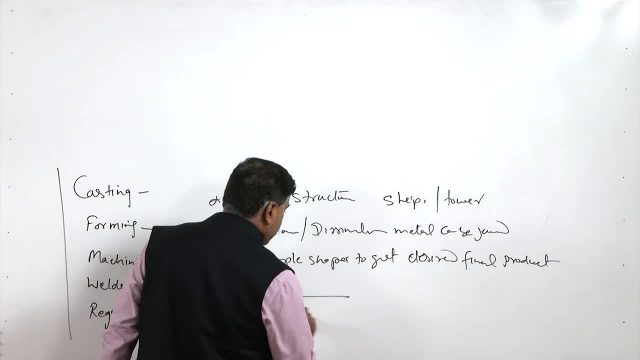 processes and it allows the joining of the similar as well as dissimilar metals. Joints can be stronger than the base metal. this is another good feature. if you are thinking that joint will be weaker, then the processes, even the fusion welding processes or the solid state joining process. they may allow to have the connection between the two, which will 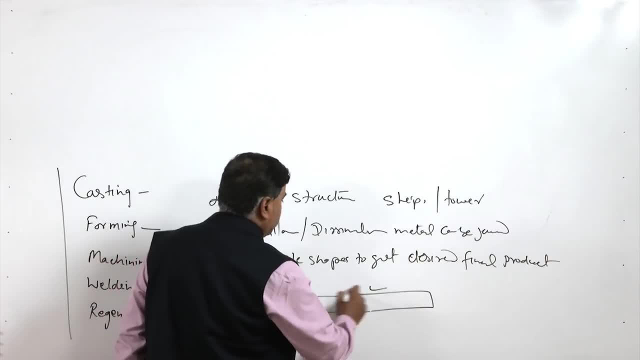 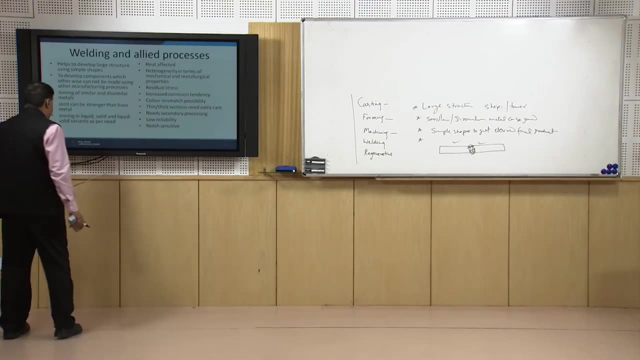 be much, even stronger than the base metal, So it will perform as good as the base metal, except that in some cases heat affected zone is produced, So that needs to be taken care of and there are various variants of the joining processes, like liquid, solid and solid. 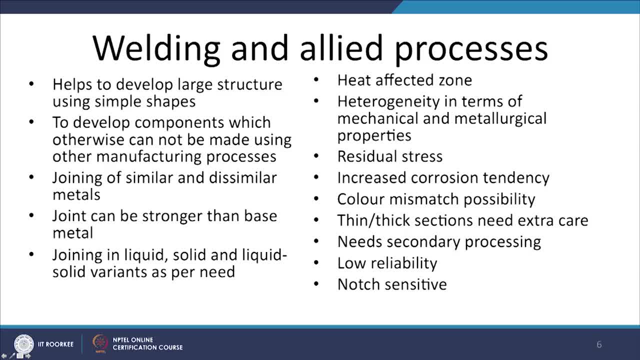 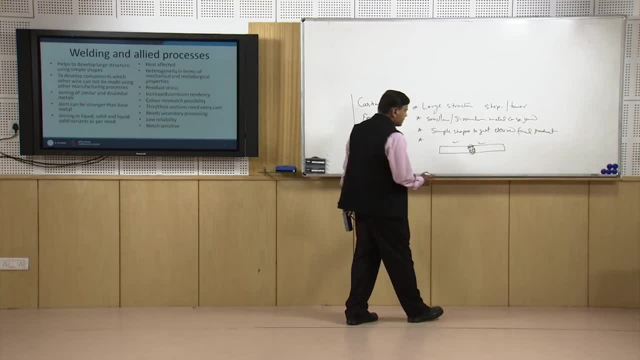 So that is another good feature. So the joint is solid and liquid, and liquid-solid variants, as per the requirement. the suitable variant can be selected so that the joint can be made. As far as the negative aspects are concerned, especially when we use the deformation based, 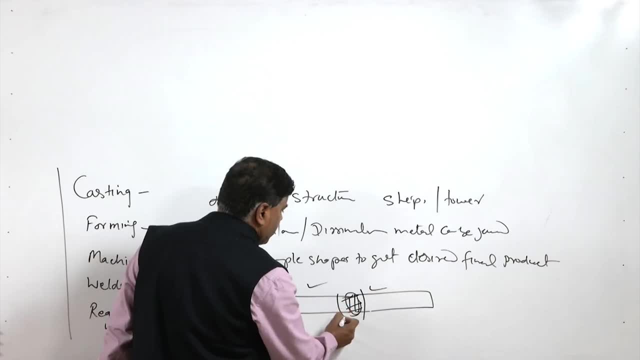 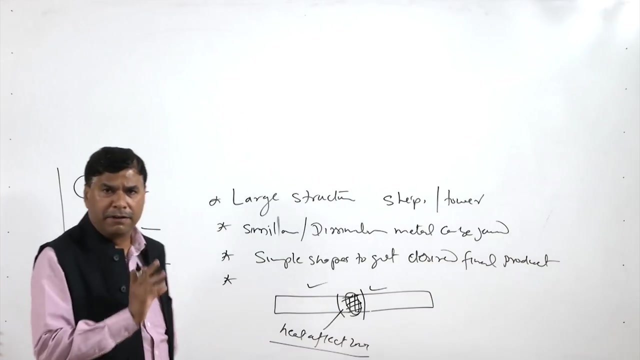 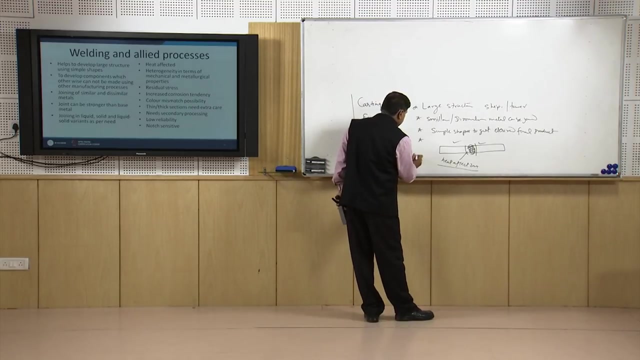 processes or the fusion based processes, we find region next to the weld joint which is called heat affected zone. This heat affected zone has the different in microstructure and different mechanical properties and therefore this, sometimes this, become the source of the weakness in the joint and therefore this heat affected zone must be taken care of. 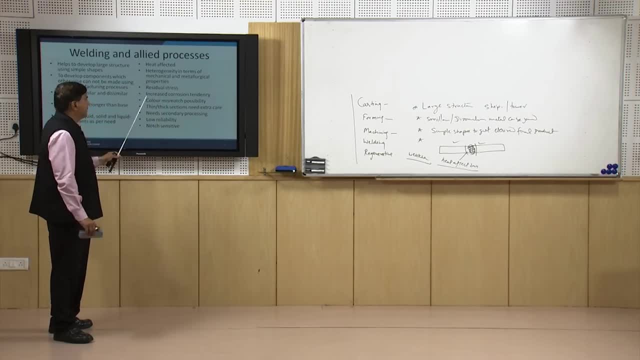 The weld joint offers the heterogeneity in terms of the mechanical properties and the heat affected zone. As I said, the heat affected zone has the different structure and different properties. Sometimes the hardening of the heat affected zone takes place and sometimes even the softening. 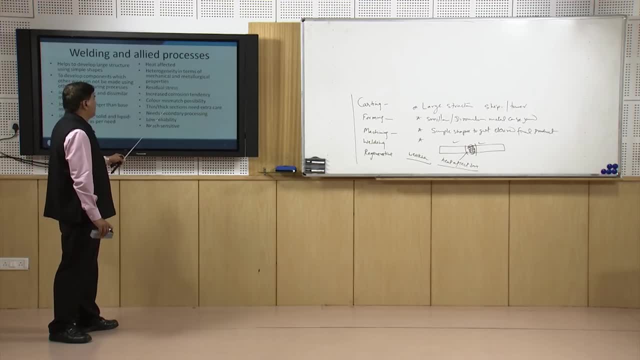 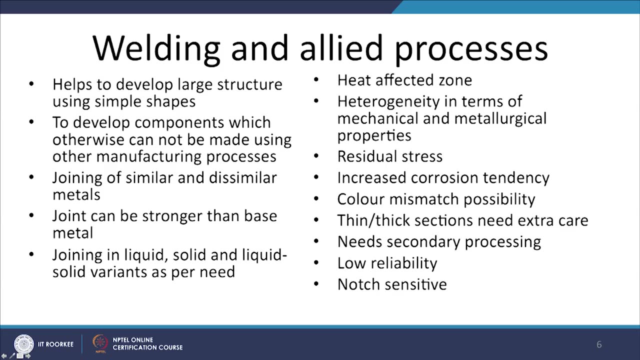 of the heat affected zone occurs. thin and thick sections need extra care. in case of the welding In thick sections, lead needs the multi pass processing which results in the very wide heat affected zone, as well as thin sections, can lead to the melt through or increase distortion. 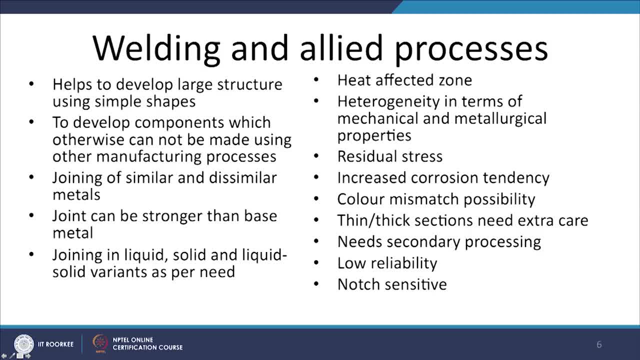 tendency of the thin sheets, The control of the weld pool becomes very difficult in case of the heat affected zone. So, thick sections, thin sections, residual stresses, which is, which are integral part of then all types of the welding processes. mostly it is found, residual stresses are found. 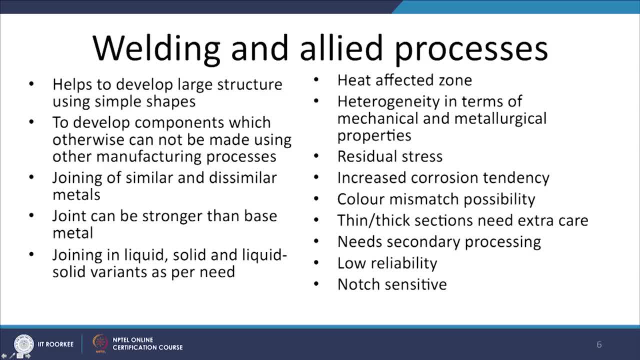 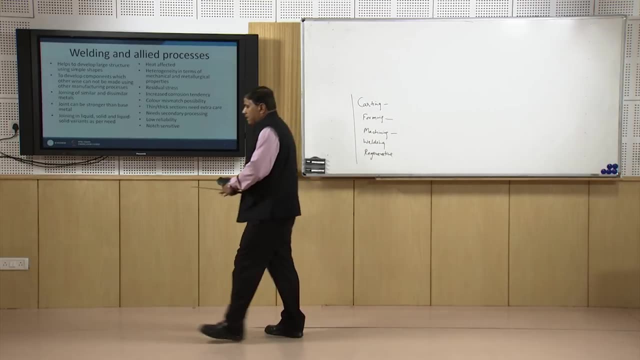 in the fusion welding processes, which are very tensile in nature, and these promote the failure in number of adverse working conditions of the weld joints, increased corrosion tendency, colour mismatch possibility and the limited reliability and no sensitivity. We know that all these features actually reduce the reliability of the weld joints. 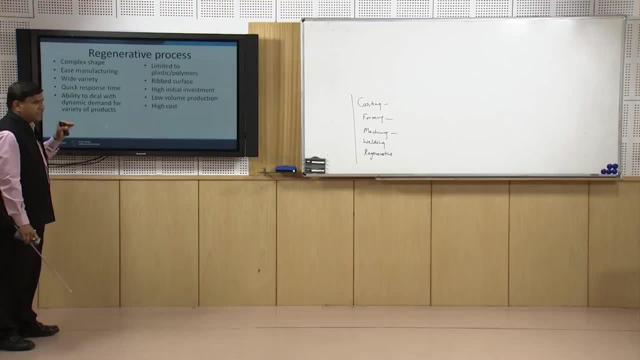 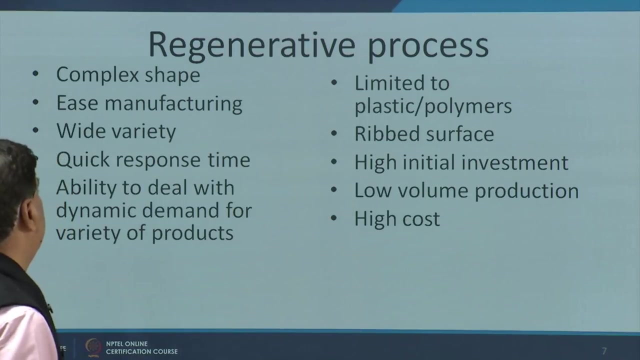 Regenerative process is another category of the manufacturing process. These are: this is the newer category of the manufacturing process where in the complex shapes can be very easily produced. This process is very easy to use for manufacturing the simple shape products of very large in variety means, the different geometrical features. 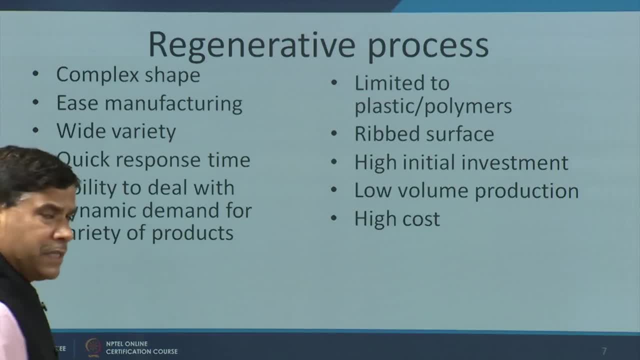 The different dimensions can be easily made because it uses the CAD, CAM and rapid prototyping principles for making the product and it offers very good response to the changing conditions of the market, So, as per the requirement of the demand or as per the requirement of the market designs. 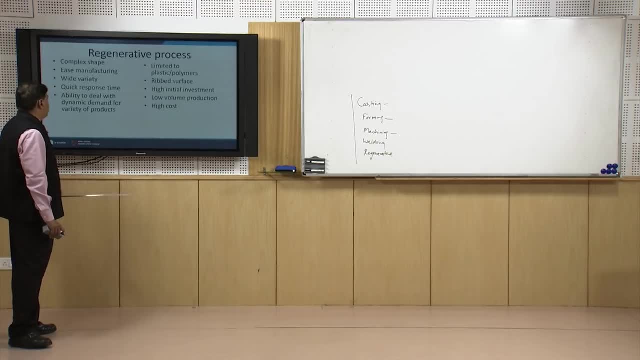 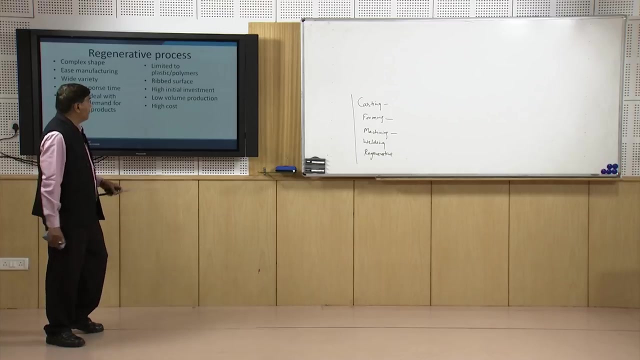 can be modified and the volumes which are to be made can be modified, although it is used for very low volume production purpose. Ability to deal with the dynamism, The dynamic demand for the variety of the products. but the limitations are like the process. these process are not very matured as of now.